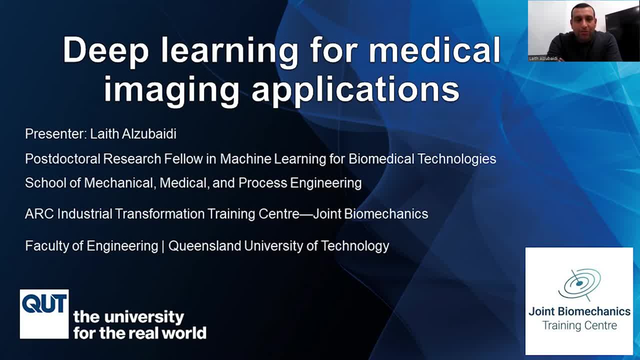 I spent, like the master's degree and PhD, working on this type of applications And during this presentation I will take you through some of the concepts, some of the challenges and solutions to that challenges and the problems and some of the ideas to think about, like. 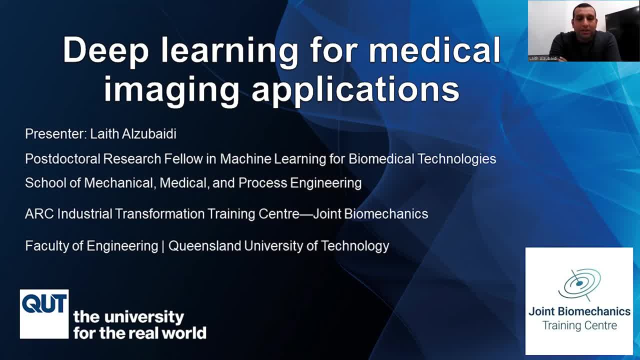 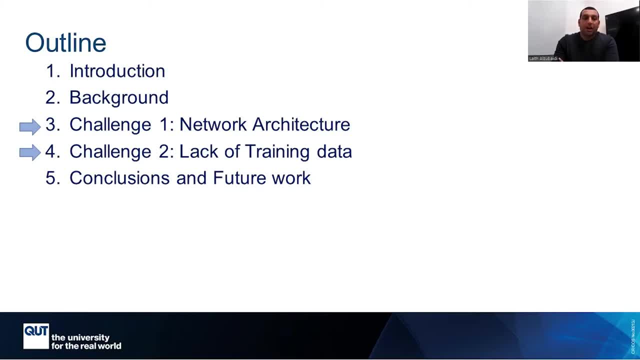 robustness, efficient like effectiveness, even explanation of the black box of deep learning. So I will take you through the introduction. background challenge: one challenge too. I will discuss two challenges indeed in this presentation: the network architecture and lack of training data. 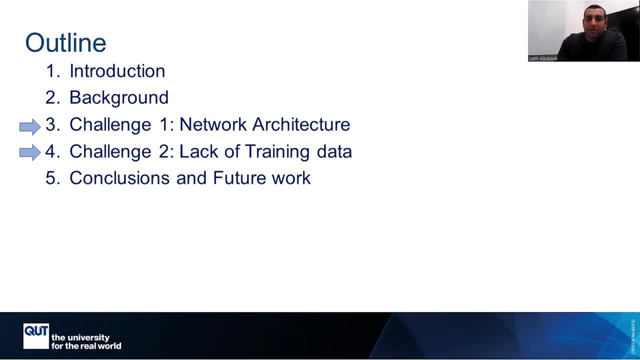 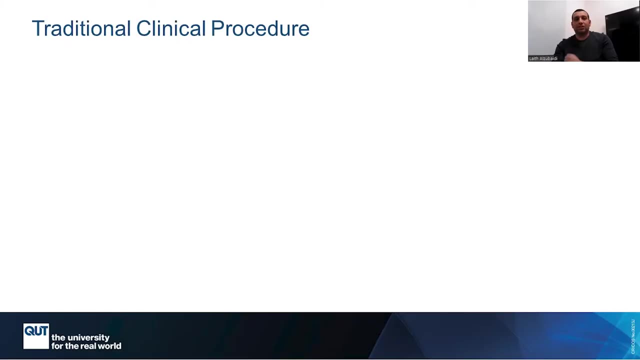 So let's get started. There are several challenges in deep learning, but these are the most common ones And these are really related to the performance of deep learning algorithms. Then we will take the conclusion on future work. So with the traditional clinical procedure, we will have three steps. 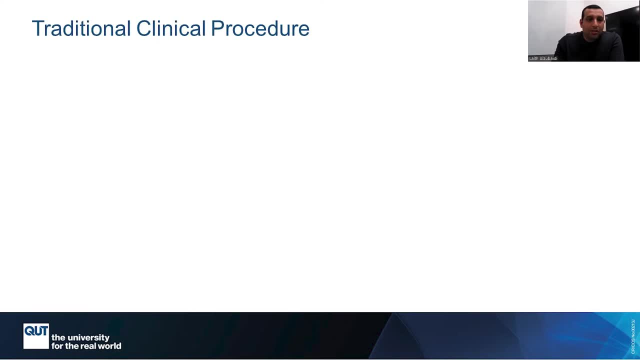 The first one is diagnosis, where we care what happened to the patient, And the second one is a prognosis, where we care about what will happen to the patient And the treatment, where the clinicians and the specialist wants to know what will give to the patients With deep learning. 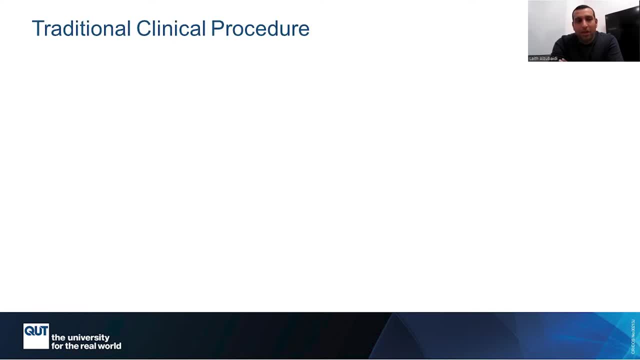 models have shown. deep learning has shown a good performance on three of these steps: medical steps And, for example, imagine. the machine will be responsible for interpretation of medical imaging, For the prognosis, like predicting the mortality from the healthcare and the predicting the treatment. 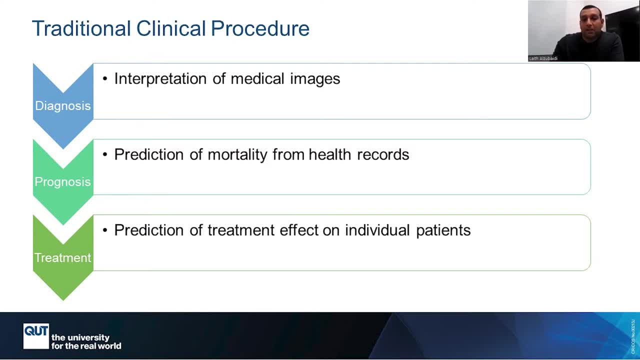 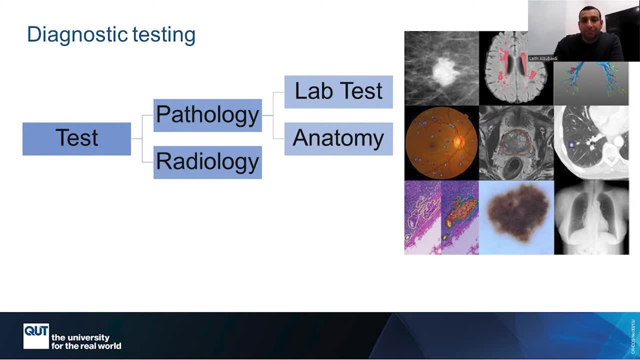 effect on individual patients. Mainly, I focus on diagnosis. That's the step where we care about and what happened to the patient. So for diagnosis, diagnosis testing, there is like pathology tests, like lab tests and autonomy and the right ology test. So, for example, with lab test, there is a 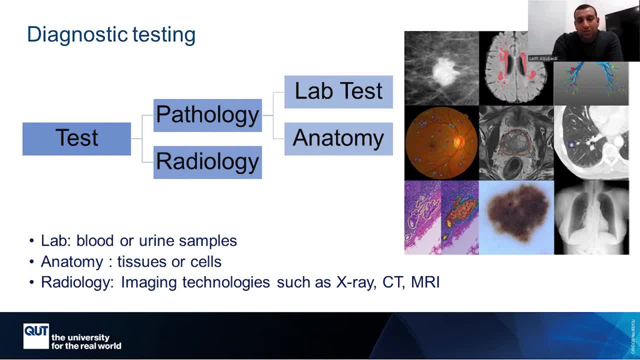 blood identity test, urine samples with antonymia like tissue or cells. with rideology. there is an image technologies like an x-ray CT MRI. deep learning has shown a great performance on all of these, like type of tests, for example on blood, like detecting from the histopology images like the. 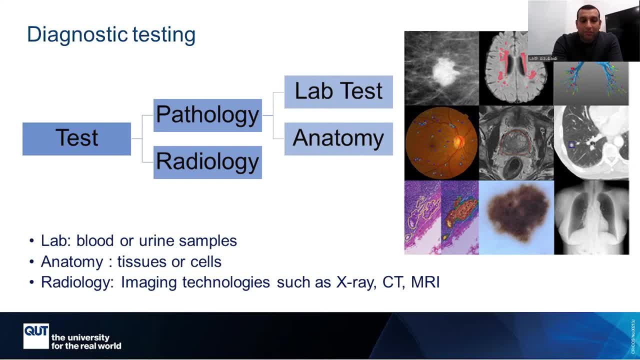 breast cancer or sickle cells, anemia from tissues and cells, as well from the imaging technologies, like an x-ray covered CT, like brain tumor, MRI, like also brain tumor and strokes- different type of diseases. so deep learning can deal with different type of images, different type of diseases. 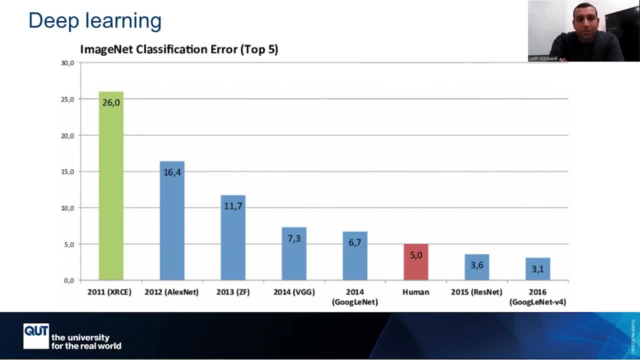 so one of the good examples of deep learning is image net classification. this is one of the famous data set that deep learning models worked on, so just like a comparison between the performance of these models, like these are the models of image of deep learning starting to compete for that data set and, at a certain point, deep learning the 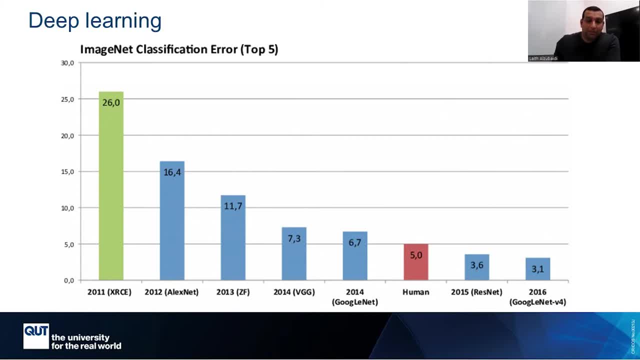 resonate model showed a performance even better than a human, which motivated people to start think about how to develop these type of algorithms in order to have a good performance. so this data set shows that deep learning can deal with 14 million images. so deep learning can deal with. 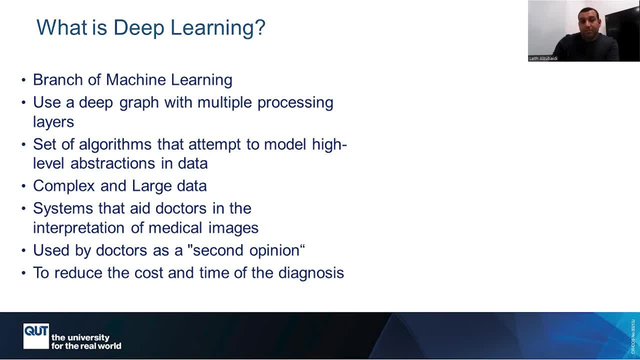 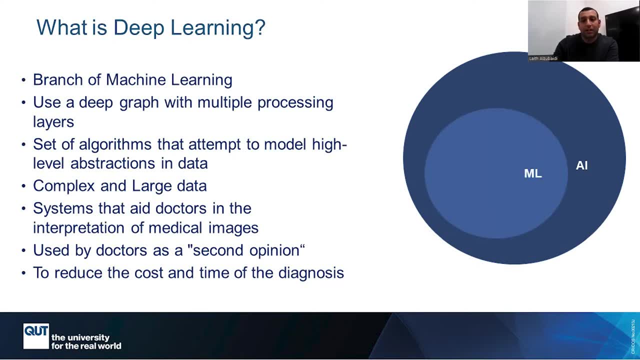 that huge number of images. so now the question is: what is deep learning? deep learning- basically the big umbrella- is AI, artificial intelligence. machine learning is part of an AI and then deep learning comes under the branch of machine learning. so it's a branch of machine learning and deep learning can deal with multiple layers, several layers that these layers have filters to. 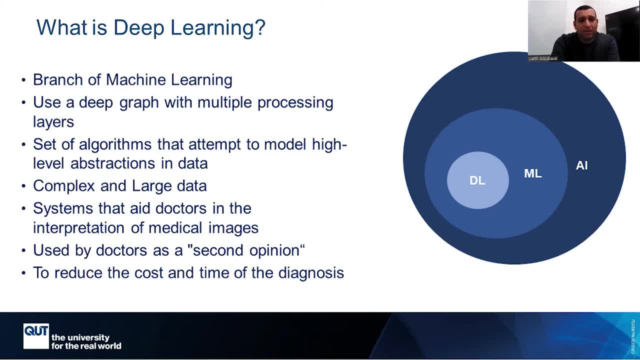 extract the features from the input image, then feed these features to the classifiers in order to do the task, whether like classification or detection, or so on. the good thing about these algorithms: these algorithms are good to deal with the complex and large data sets, and these systems of deep learning help in 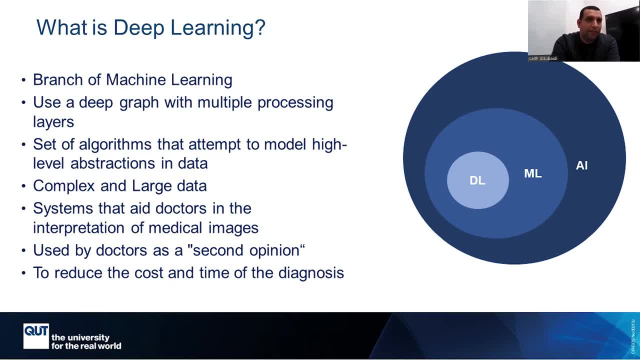 terms of giving a second opinion to the adapters, like having having like two opinions on on a task or on a case is better than better than having one opinion. so these algorithms helps in terms. these algorithms help in terms of reducing the cost, the time of the diagnosis, 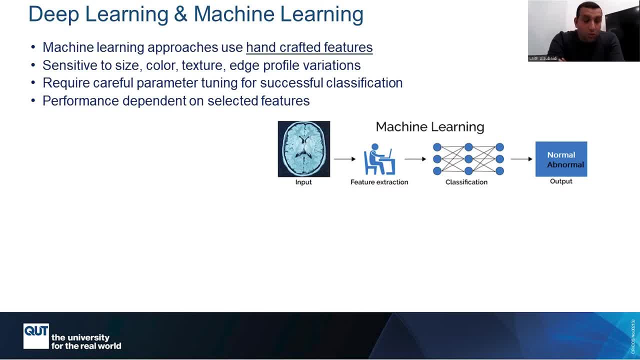 so one of the main questions that I usually receive: what is the difference between machine learning and deep learning? so imagine this scenario: when we have the, for the long time, machine learning, the traditional procedures, there is an input image and then there is a guy who is responsible to extract features. what do I mean by features? 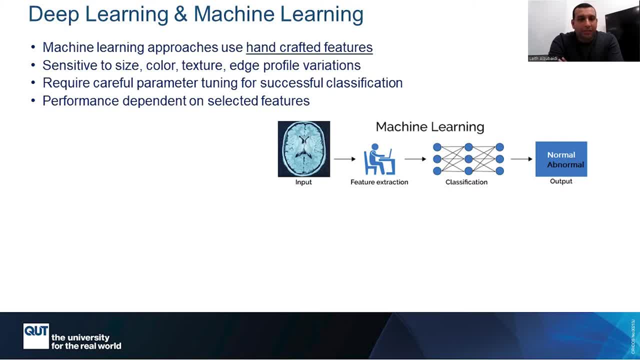 features means that that person will go, for example, in case of medical images, to the specialist and tell them: hey, what's, what's make difference about this image? where do you look what's important about that image in order to make the decision? for example, say, the shape or 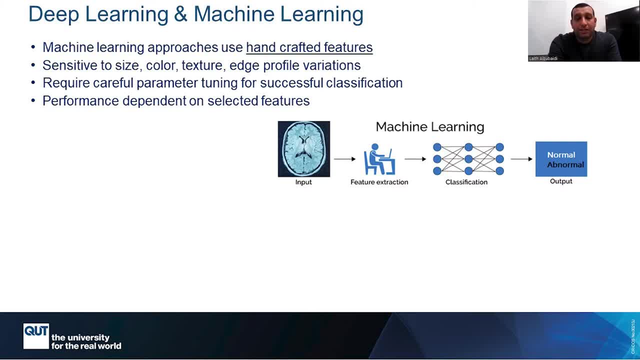 the textures or the size or the color and then, based on that, that person will extract the features, will design a filter on top of an image to extract the feature based on what he was told, and then extract the feature and feed that features to classification to learn from that feature to do the output. 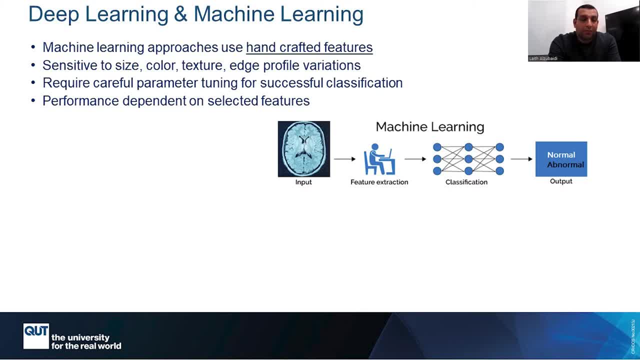 so one of the problems of that, so the performance will be based on that feature extraction. so it could be not the right features to discriminate between classes. it could be biased to something so that performance could be even like not having a good ability to deal with large amount of data, different scenarios, like complex data, in order to extract all relevant. 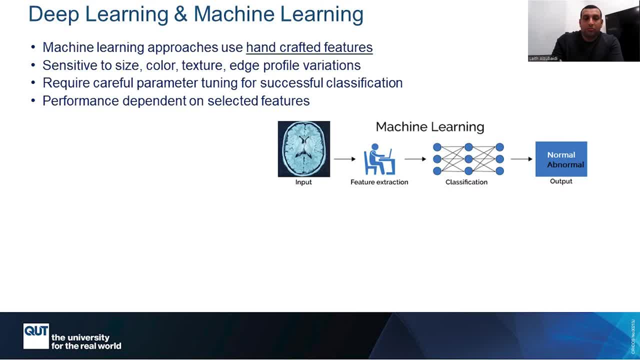 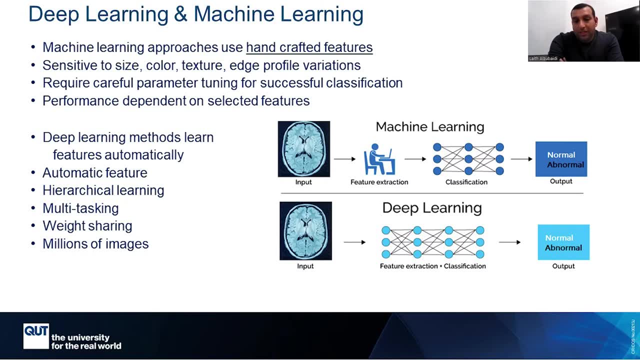 features in order to do the classifications. so later on, deep learning came and showed that ability to do both of these- feature extraction and the classification- in one shot, like just doing the classification, automatically doing the feature extraction and the classification at the same time, without designing any algorithm for feature extraction. so deep learning learn the features. 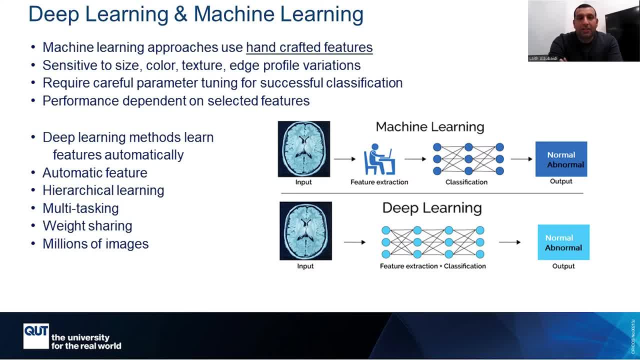 automatically and can deal with the several tasks: million of images, just like we saw for ImageNet dataset, so showing a really huge ability to deal with the classification, for example. but the problem again with deep learning requires large amount of data in order to learn from that input data. 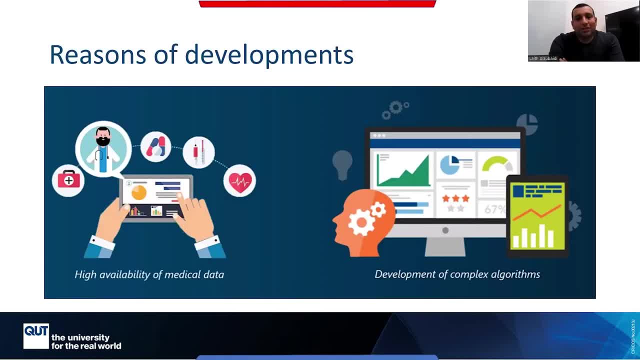 so for the reason, the reasons that just this deep learning appeared and starting to take the role of doing many tasks currently: high availability of medical data, starting the data to increase and showing a huge amount of data around the world. development of complex algorithms, these algorithms from deep learning starting to develop and getting. 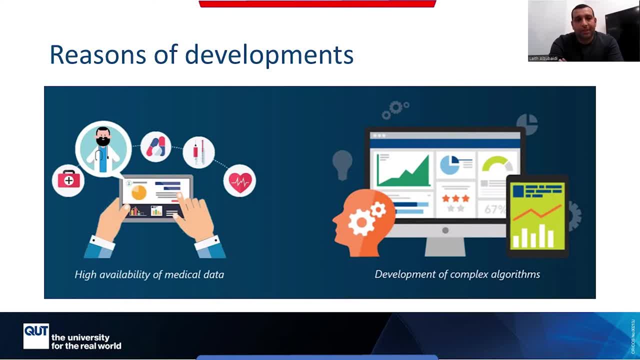 what we're calling high application training: mining and also the use of the machine and how to do using these algorithms. and it's smart that deep learning is really good in a way, how to deal with the medical data and also, i personally believe, because of the high computational tools. 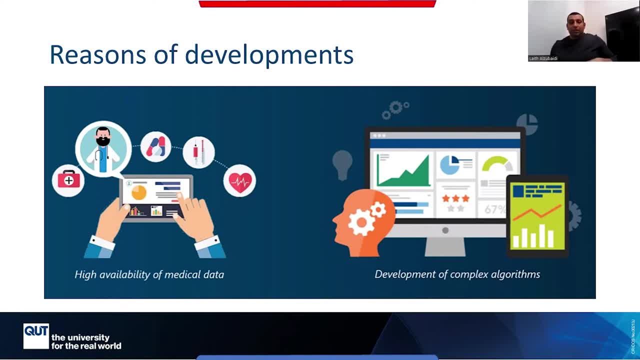 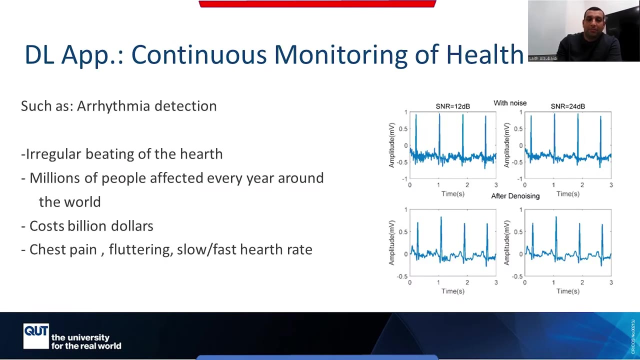 that we have currently to train these algorithms, so for very long time, machine learning, uh algorithms able to do that and to handle these. I mean the complexity with the, along with the computational tools in order, like, for example, GPUs, TPUs and so on. so some of the examples of that. 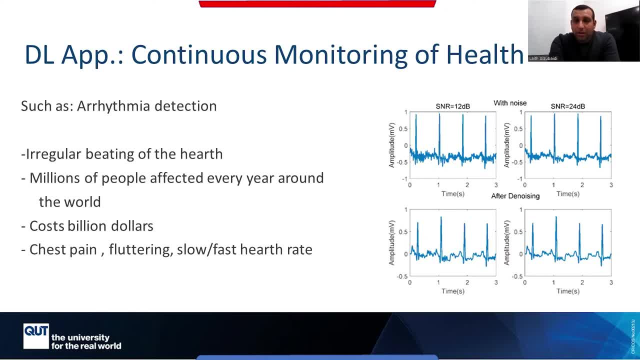 deep learning applications, continuous monitoring of health- for example, arrhythmia detection, one of the good examples- like monitoring millions of people around the world affected by that can just reduce the cost and, the most important, can just predict what will happen to the people with that problem and tell them. tell them exactly like, for example, based on the record. 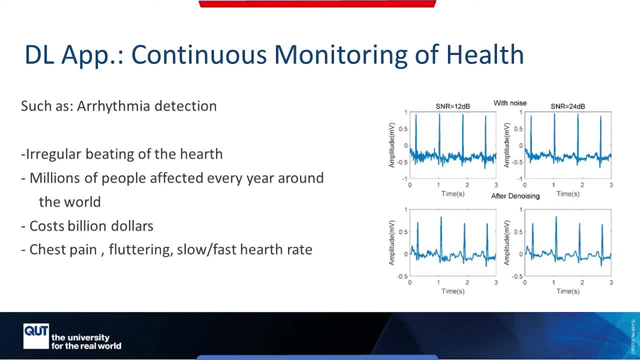 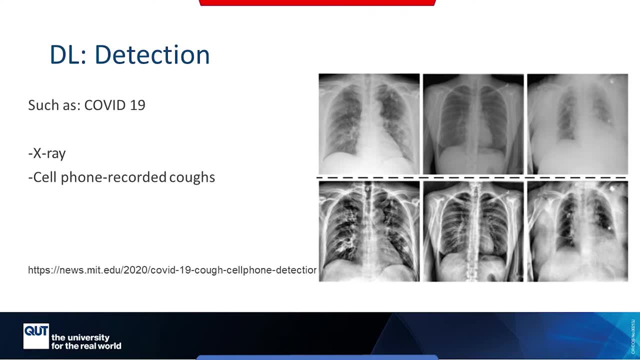 and the heartbeats, then they are able to predict something and save lives. another example is COVID detection. several examples like algorithms worked based on x-ray images to detect whether there is a COVID or not, and even they used a cell phone application to record the to classify the. 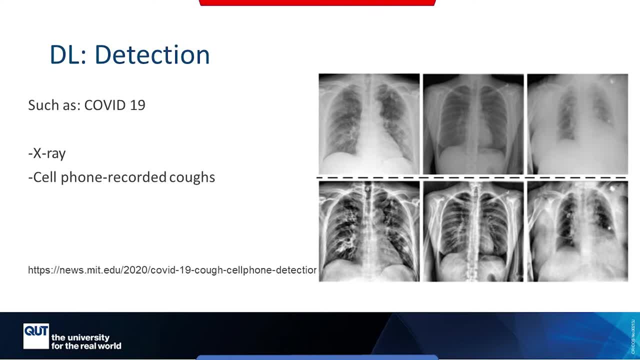 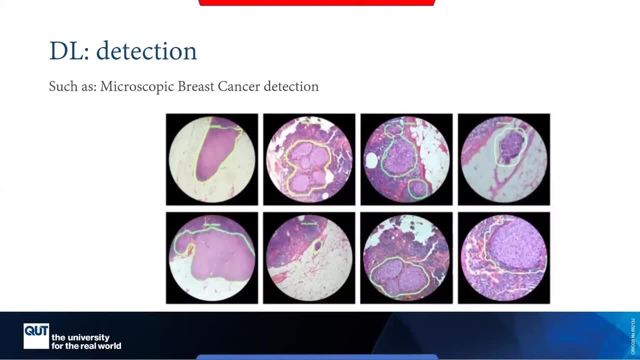 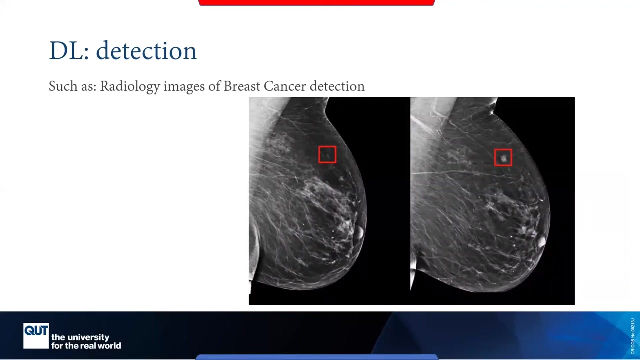 COVID versus non-COVID based on recorded cops. so by just using the application to do that, which is really great. another example is microscopic breast cancer detection. deep learning is showing great performance on that. applications breast cancer detection as well. at the very early stage. deep learning showed a huge performance on that by just detecting the 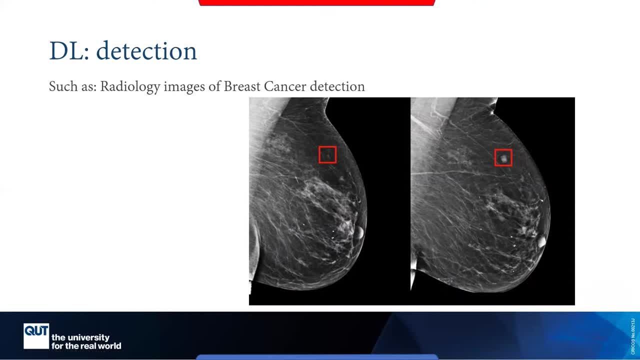 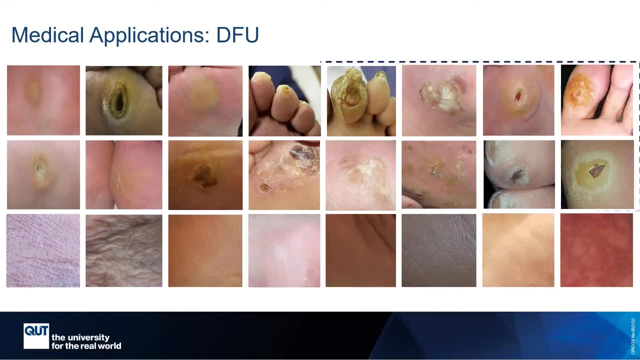 breast cancer from very early stage based on their ideology images. another example is DFU diabetic food, also classifying whether it's normal or abnormal based on the umbrage image of that foot and telling whether it's there is a problem or not. or there is maybe a DFU or not compared to the wound or different type of. 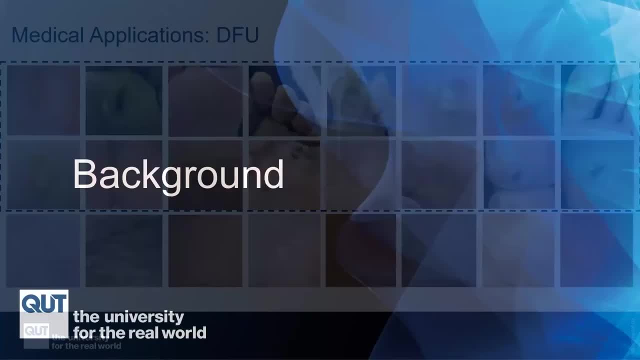 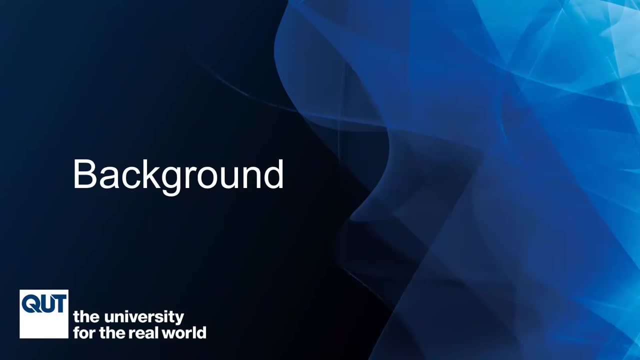 injuries in the foot. so showing these are what we learned from- that arms like the deep learning can really show huge performance on medical images. before we dive in the details, I would very quickly give introduction. maybe we can answer the questions later on when we finish. so the background. I would start by so giving very quick background about the machine learning. 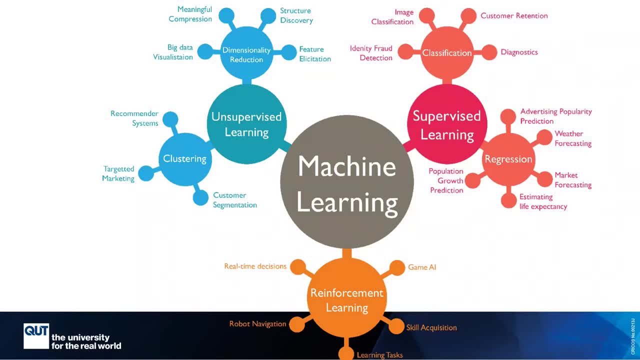 in general. so in order, I'll give learning and machine learning in general. in order to deal with these algorithms, we need to first figure out which way we are dealing with or which path we should go with. so there is supervised learning, whether you want to do classification, for example, diagnosis- 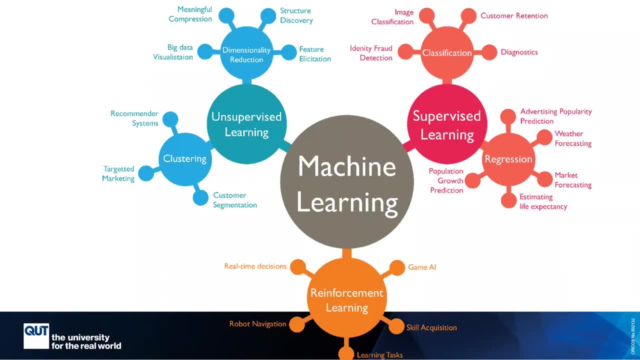 imaging, classification, different applications where we have the label, like there is an input image and there is an output, a layer or, sorry, a label that matches with that in input image, for example, I have an image of MRI, then definitely. for example, I have the normal and abnormal labels with the recreation. 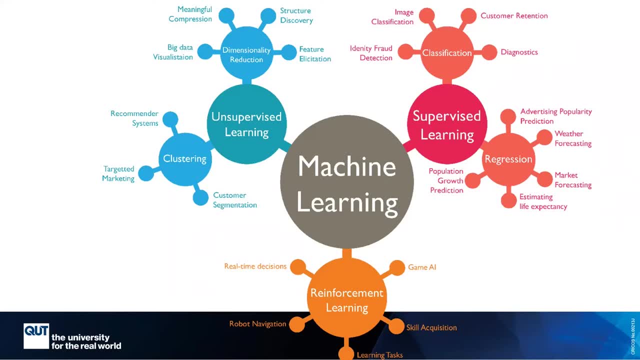 as well, like we predict, for example, whether forecasting, market forecasting as well, on different applications where we predict based on the data that we have and supervised learning, like we don't have the label but, for example, of clustering, dimension, altering production, there is reinforcement learning and there's other type of learning. 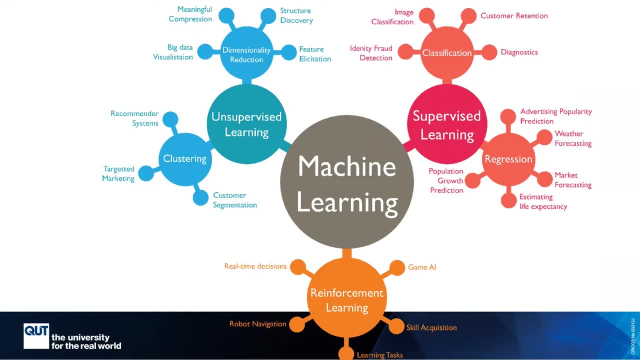 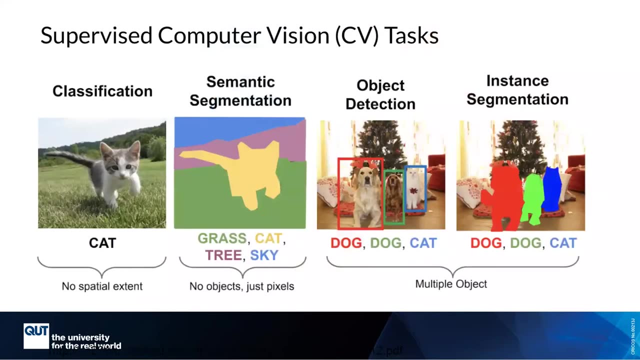 so, before we go ahead and start these algorithms, we need to know which type of data, which type of a problem that we're dealing with. also, for example, we decided to work on supervised learning, for example, computer vision task. do we need to do like? think about you want to do the classification task or semantic? 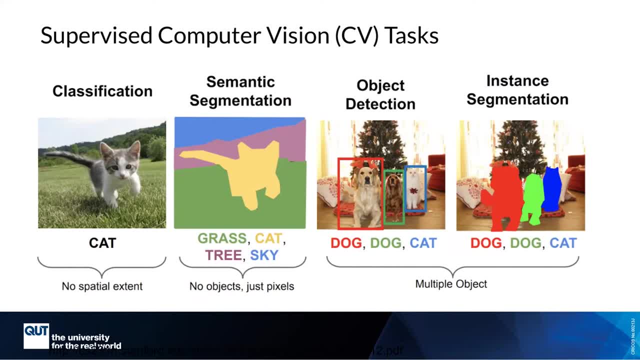 segmentation, object detection on instant segmentation. so basically, based on that, whatever that you will work on, for example for medical images, you need to think about how to prepare your data for that task. for example, with the classification: we just say: what is in that an image like, what's in what type of object in that image, for example, the cat? we say there is a. 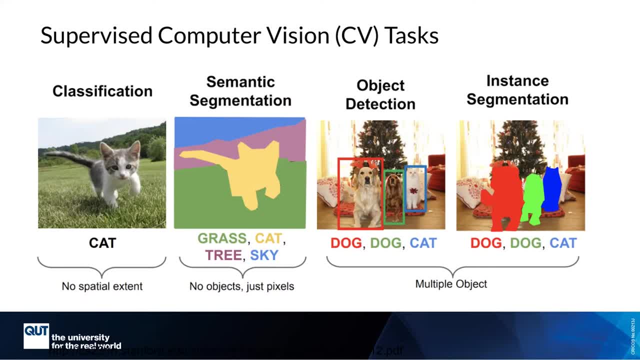 cat. so I already prepared the classification by having the image on the label of each of these images to train the deep learning model for segmentation, for example, I have the mask for that, so I need to feed the neural network with the mask and the original images with the object detection. for example, I have the object on the 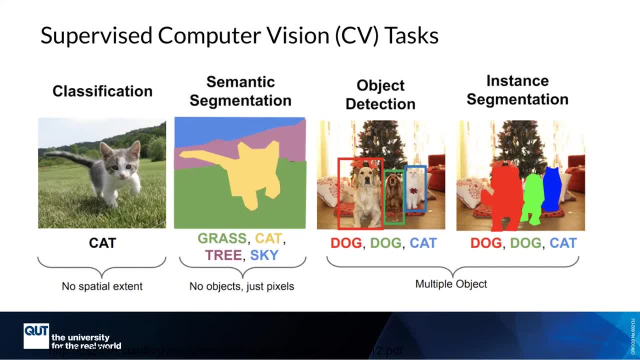 boundary box for single images, like images that I have in order to train the deep learning models, and, with the same thing, with instant segmentation when I have the mask for the object in the image. so, again, based on the task that you will work on, then definitely you need to prepare data based on the task. so, as you see here, 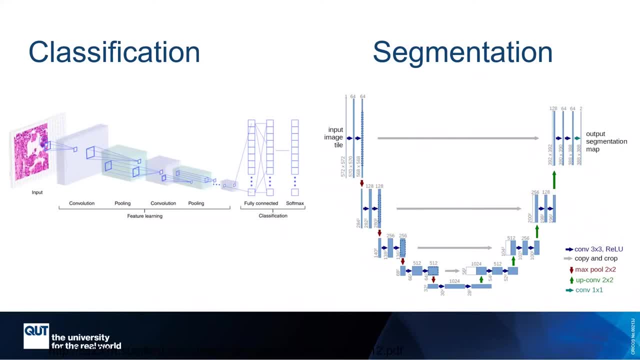 again, if you decide for classification, there are specific application. I mean algorithms, deep learning algorithms for classification, for example convolutional neural network. this is one of the most popular one for deep learning algorithms or models. if you decide segmentation, for example, maybe you can use unit and other application or other algorithms, or maybe you built your own algorithm or model. 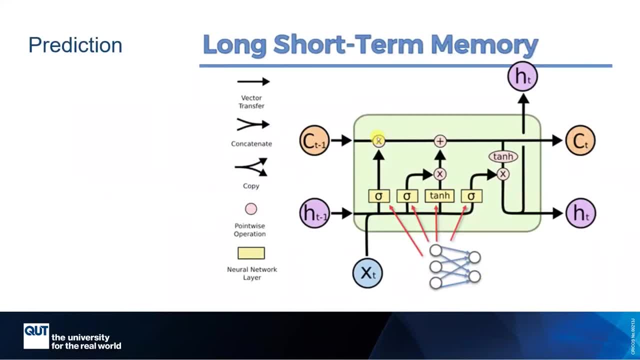 maybe for a prediction, there is long, short term memory to use. the purpose of mentioning that is to show that, based on the tasks you will work on, you will decide which direction and which way you will work on, which type of algorithms you need to look for. so the general 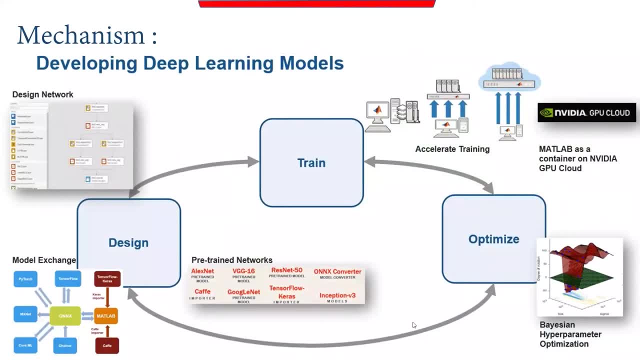 the general mechanism of any deep learning model is based on you first design your own network or you use some of the existing models like AlexNet, VGG, ResNet, GoogleNet, maybe TensorFlow, itorch, any library, to import these models. you may design your own model and then you go through the 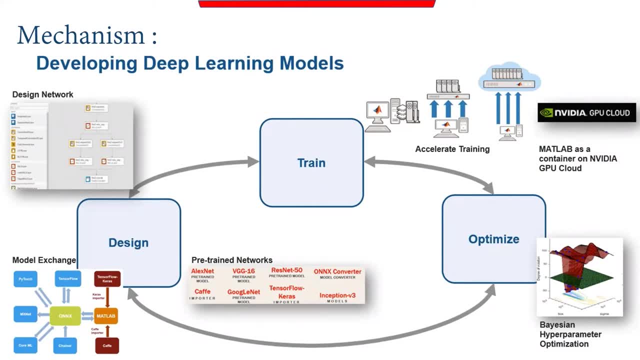 training first, and you define the data set by the system and then you start the model roadmap and it based on training and testing and validation as well- um, we'll explain that later on- and then you optimize. you pick the training parameters, optimizers on the learning rate, ebooks, iterations. 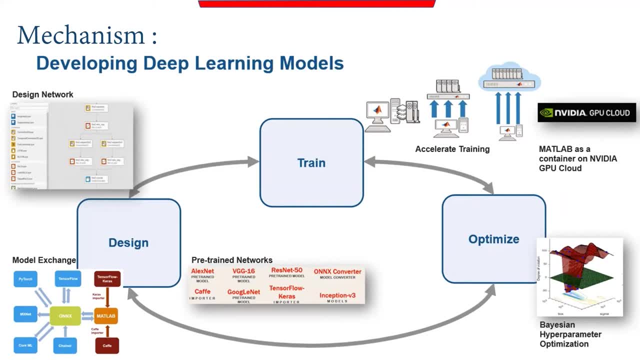 all this type of setup in order to train the deep learning, optimize it. if you get a good performance, then you move on, if not, you go back and you modify the design and do the training again. that's kind of the procedure, the whole mechanism of any deep learning model. 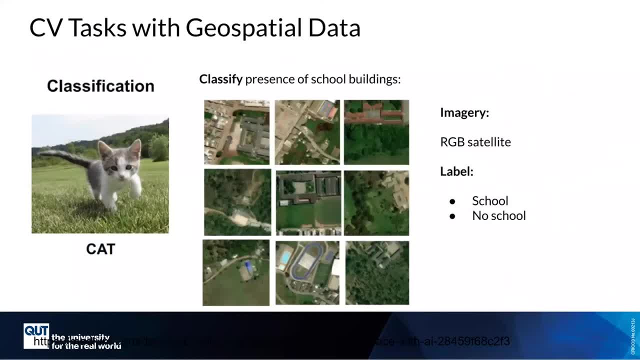 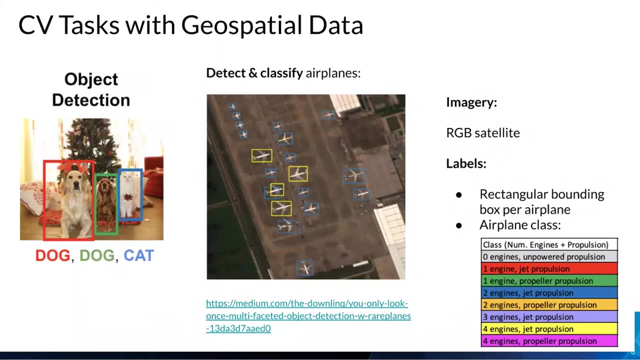 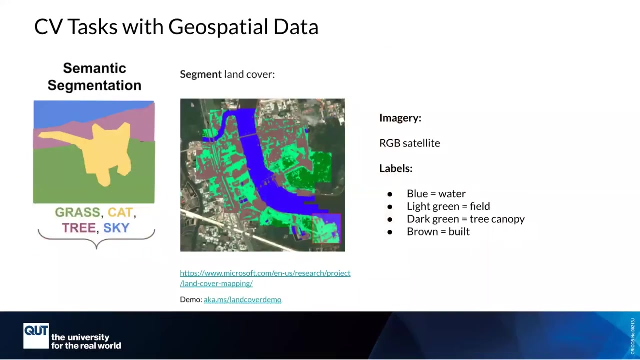 so uh, very quick example, another example of classification: for example, we have an image of an uh satellite, rgb satellite, whether it's in school or not. school, for example, with um, with the object detection, where we detect some, for example the boundary box, the airplane with the one engine or two engines. where we have another image where we say um, this. 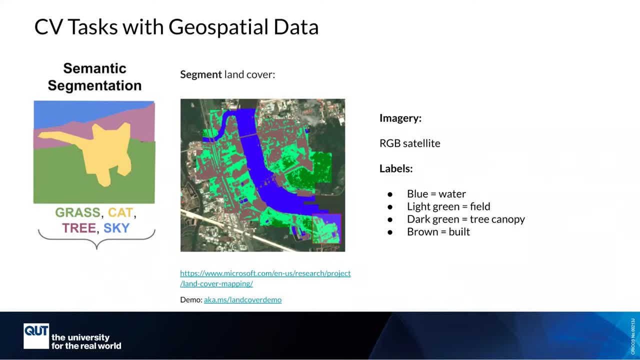 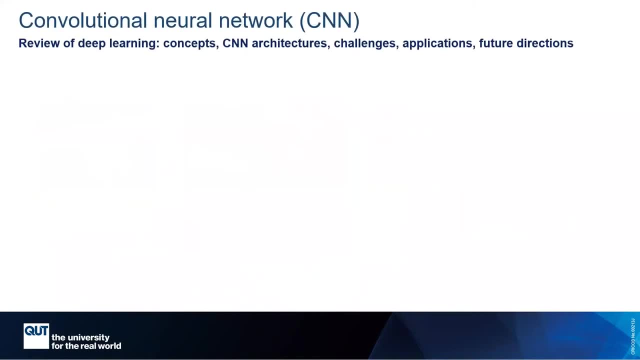 is this blue area is a water, and this light green is a field, or dark green is a tree, and so on. so it's kind of specifying the area, um of this application. i'm trying to show several examples, not just only medical images. so, based on the literature, one of the good examples of 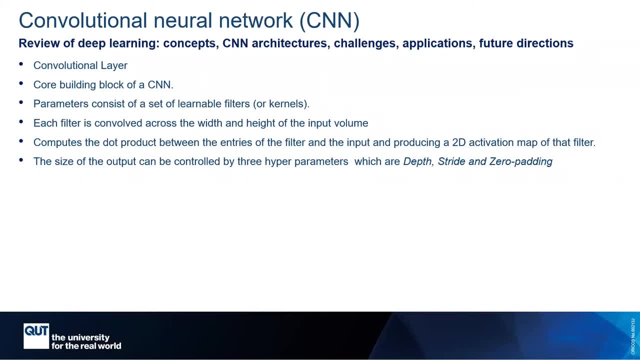 of good algorithms and deep learning is popular because of this algorithm, which is convolutional neural network. this algorithm is mainly used for classification, different applications of medical images. so previously this algorithm is based on- there is an onboard image- will go through several layers in order to extract the features and, uh, one of the features called convolutional feature. 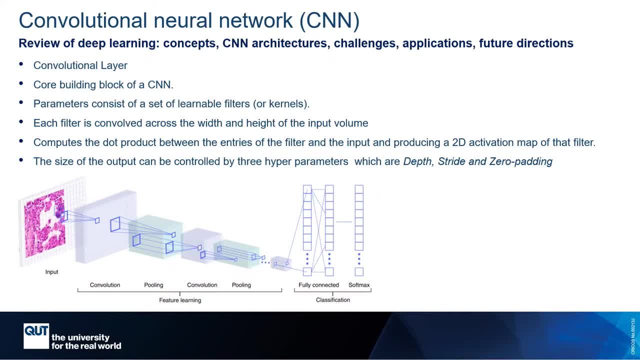 a layer that is responsible for extracting the features. there is several parameters in that layer: um. in that algorithm showing the depth is tried and the padding could be zero padding or not. and there is another um layer, which called um, so that that convolution layer has a filter, will go through the image in order to get. 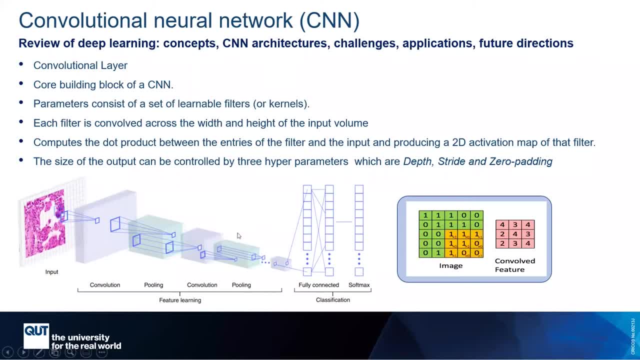 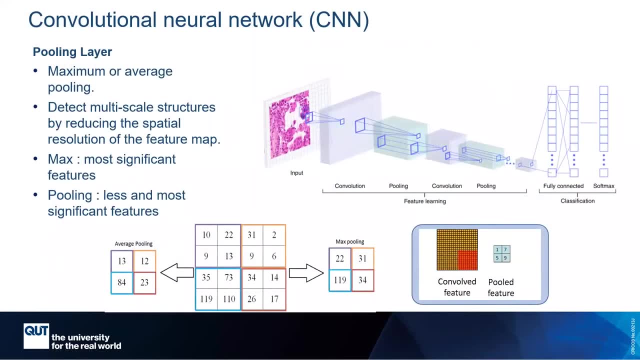 the feature, extract the feature. then there is another layer called pooling layer, where the starting to reduce the dimensionality of the onboard image. the purpose is to get one uh array. like to pass it to the fully connected with each of these arrays will uh represent one of the input images? 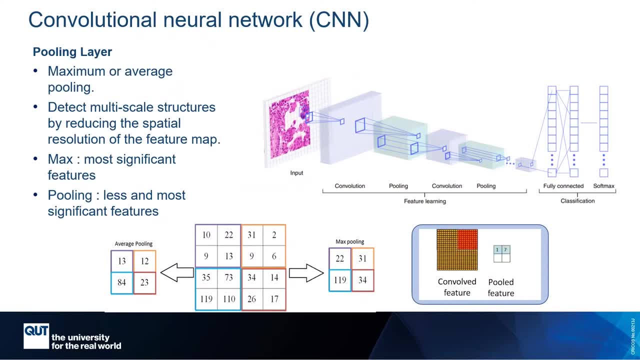 to uh train these fully connected layers and come up with the probability of the classes that will classify, and we'll see different examples, several uh ways, several types of that pulling there. for example, average pooling, maximum pooling. there is even global average pooling. um, there is uh a global 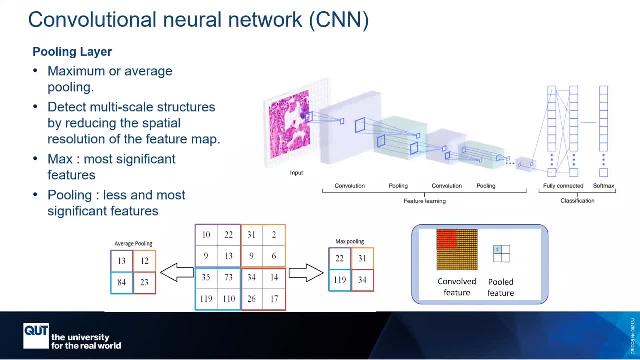 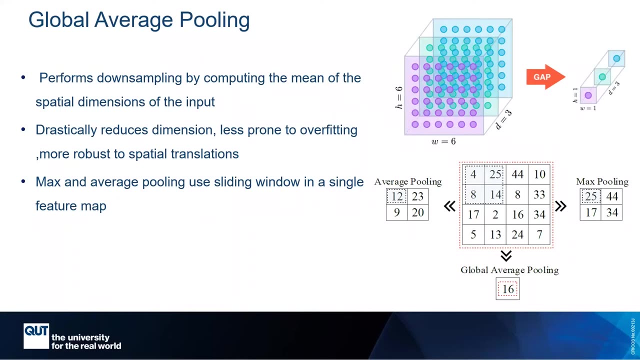 maximum pooling. there are several details with these algorithms. i'm just going through these very quick um. if you want to look more, maybe in the future to have more details about that in different webinar. one of the good examples again is to reduce the dimensionality and dealing with 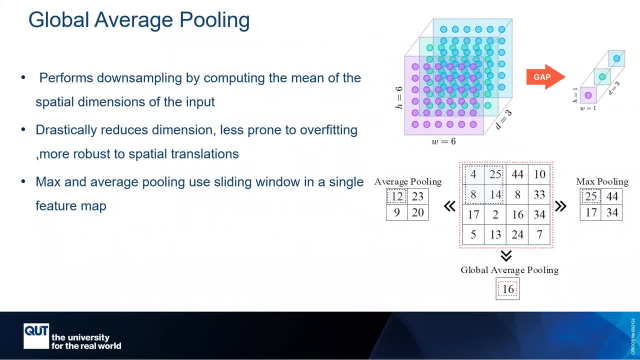 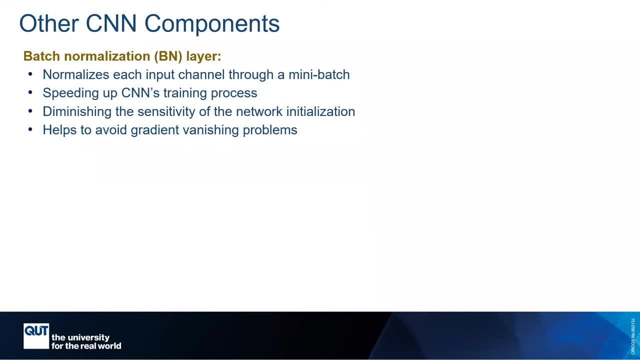 these things is global average pooling, where take the whole image and reduce it in one single bit. another component of that cnn is patch normalization, where we normalize the output channel from minimum batch. this kind of layers helps in in terms of speeding up the cnn training process and even helps in avoiding reading flash problem, and we'll talk about this problem. 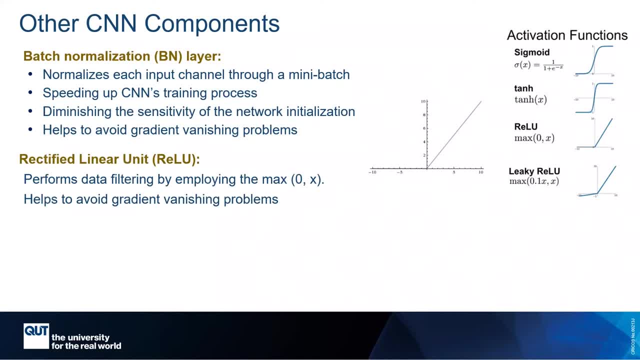 later on, like tanh, rectilinear unit, sigmoid, and one of the good ones is rectilinear unit, which helps in order to avoid also gradient vanishing problem. There is another type of layers called dropout layers, where the neurons are randomly turned on and off in order to avoid overfitting. 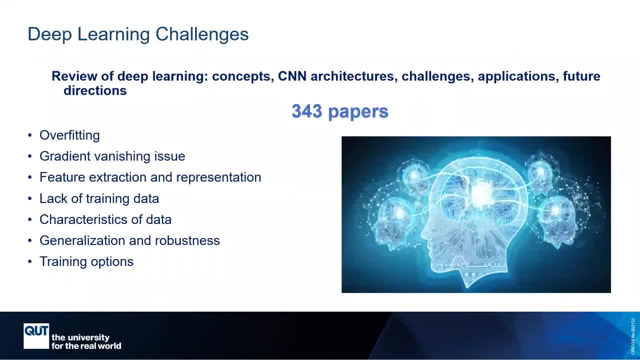 So, based on the review that we have done in this paper of review, deep learning concepts, CNN architectures and challenges: applications: future direction, we came up with the conclusion of: we can conclude the problem of deep learning in three different ways. The first one is based on the structures, which are the overfitting gradient, vanishing issue and feature extraction and consultations. 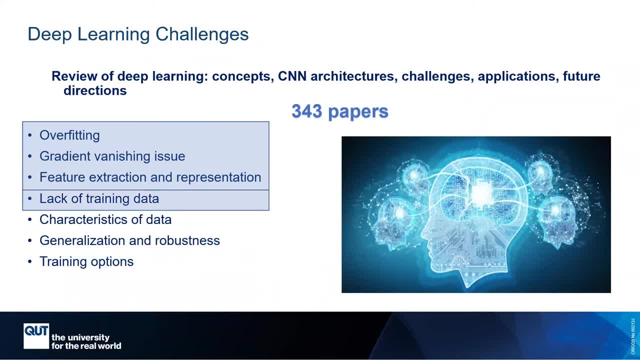 The second part is the lockout. The third one is how to deal with different characteristics of the data, how to deal with the robustness and generalization, how to set up the training options, like which type of optimizers to use or which type of learning or activation function to use. 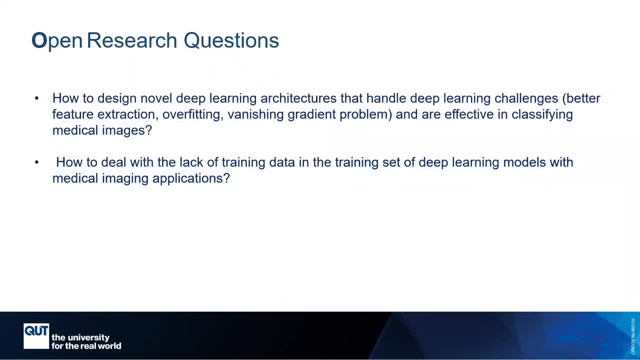 So that can lead us to two main open research questions. The first one: how to design the deep learning architecture. The second one: how to design the deep learning architecture. The third one: how to design the deep learning architecture. The fourth one: how to design the deep learning architecture. 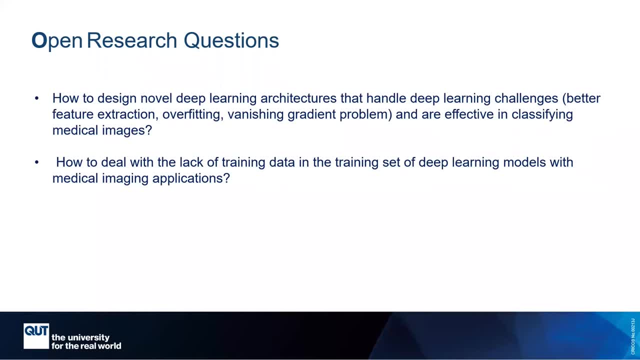 And the last one, how to design the deep learning architecture. So these are two main questions that can deal with these problems of feature extraction: good feature extraction, overfitting, vanishing gradient problem and so on. for medical images: 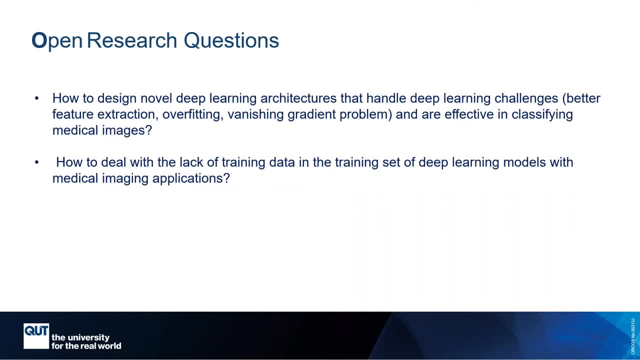 And how to deal with the lack of training data, How to come up with a good model that trains well on large amounts of data, while it's really hard for medical applications to get large amounts of data. So this is a great question. So we'll go through the first challenge, or the first research question, very quick. 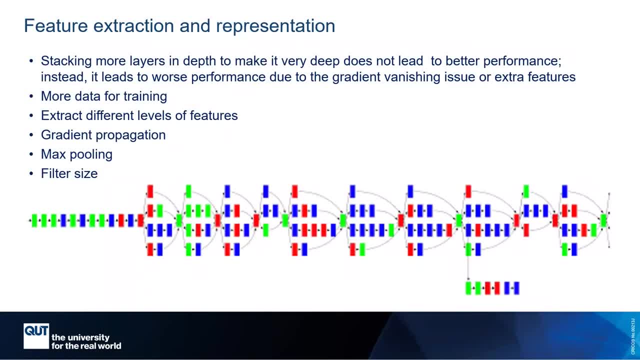 The main problem with that is how to design a deep learning model. Do I need to have a shallow model? Do I need to have a very deep model? Personally, I believe it's based on the data that you have, Because having a very deep model will lead to a problem of overfitting. 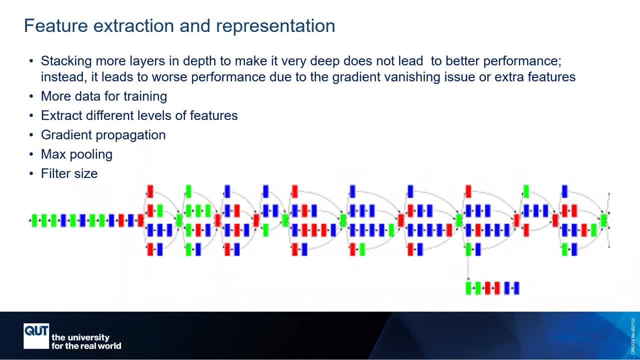 Definitely, if you have a small amount of data, then you need to think about the depth. However, if you have a large amount of data with a very complex, definitely more layers in order to learn more about these images, extract more features to do. 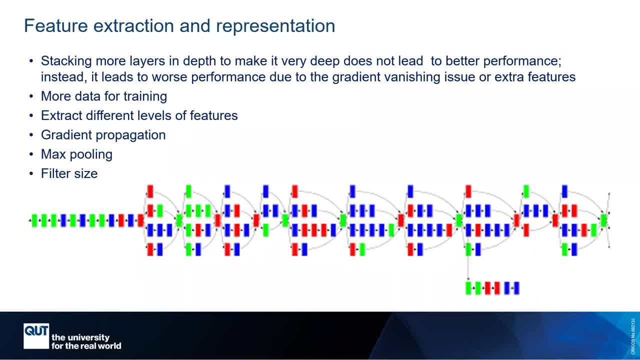 Traditionally, many algorithms and models use just the- they call it plain or one-dimension model- like layer following each layer, There is a. There are multiple layers that follow each other. The problem with that? that will lead to, for example, having one filter size. 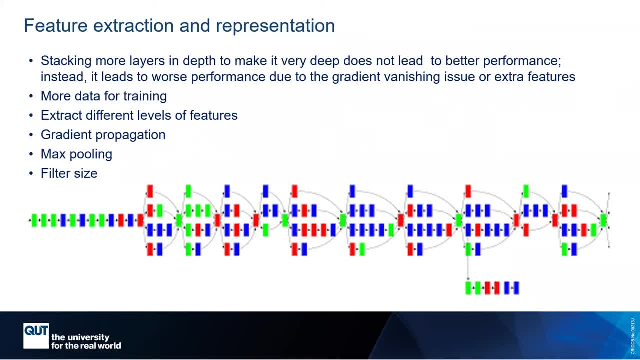 Like having one filter size. If you go with a small amount or a small size of filter size, like one by one, then that means you will extract the big small features and ignore the large features or the shapes It will give like a narrow point of view. 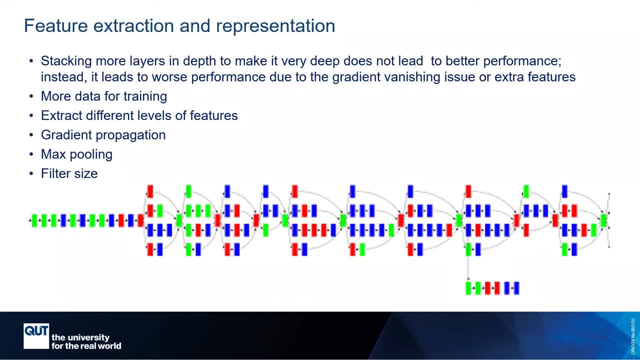 However, if you go with a big one, Then you ignore The network, will ignore the small ones. One of the good techniques to deal with that they call it parallel convolution. As you see here, several models recently, like GoogleNet, Ception, Exception- all these type of models were designed based on parallel processing. 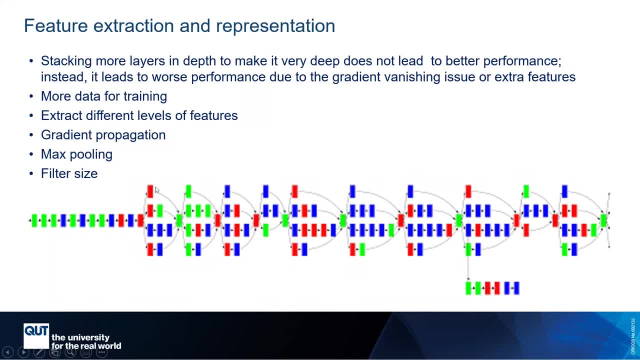 where there is several layers that work together with a different filter size, like starting one by one and three by three, five by five, seven by seven, then so on, and then combine all of that in one layer and then feed it to the next block in order to do the same procedure. 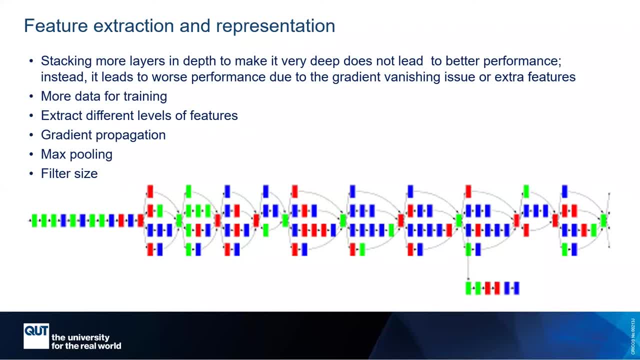 which this technique helps in a way that can extract different level of features, like different types of features, and at the same time, help with the gradient provocation, as the gradient will just use several paths in order to maintain that gradient. Okay, Thank you. 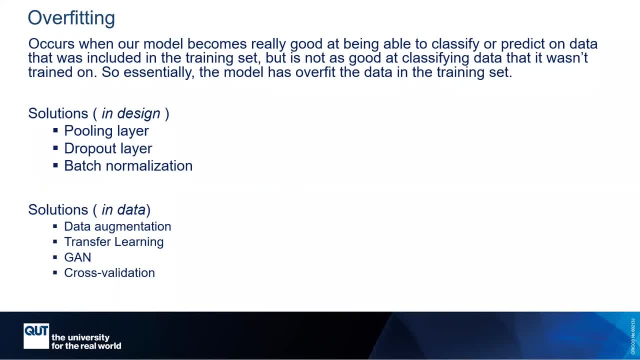 Another problem is overfitting. Overfitting means that the model learned the data very well. Usually this problem will occur when we have small amount of training, Like the model. usually this is one of the biggest problem that I ever witnessed with many people who work with deep learning by just thinking you have a small data set. 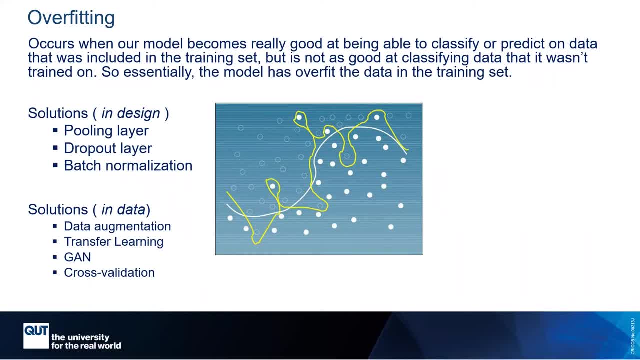 you tested that model, oh, I got 99% accuracy and I'm good. Okay, I'm good to go. Then, when you move on to the real world and test your model on different data for the same task, you will get surprised that the model showing a really bad performance on that. 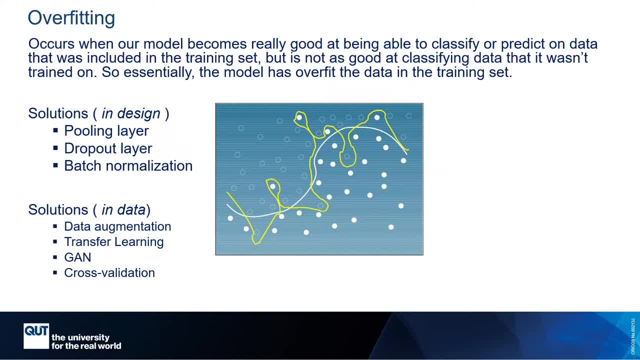 That means the model learned the specific data only for that data and is not able to classify other types like different data. So how to deal with the problem? And there's different directions. The first one: Okay, This is a problem that you can do from the design's point of view by using the pooling layer or drop out layer, batch normalizations. all of these three help in terms of overfitting. 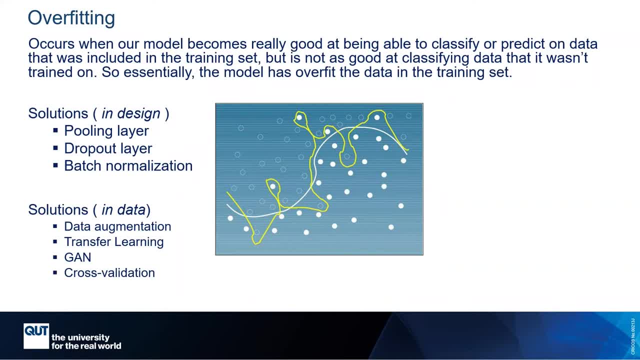 Another problem. Another solution is to increase the data set in order to deal with that problem And having several scenarios in order to deal with that. For example, data augmentation using several types of data. There are several types of data augmentation: validation or transfer, learning, GAN to generate more data. cross-validation can help in this. 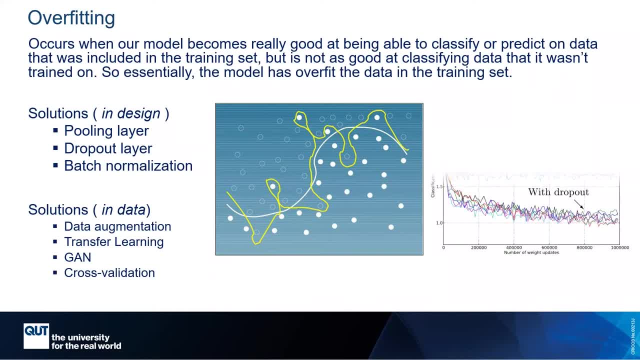 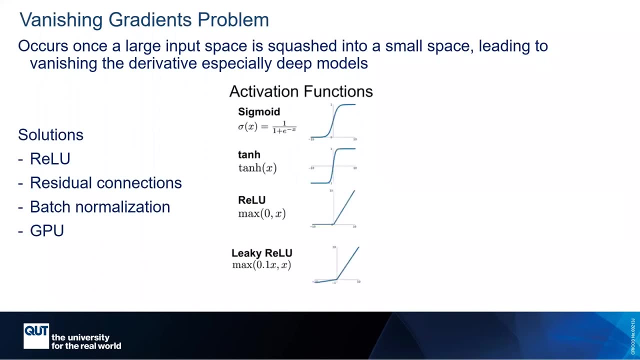 problem also to get rid of that, And this is example of showing where to use the with and without the dropout layer: how the error just got reduced by using the dropout layer. Another problem is gradient vanishing problem where there is a sigmoid tan-edge rectifier. 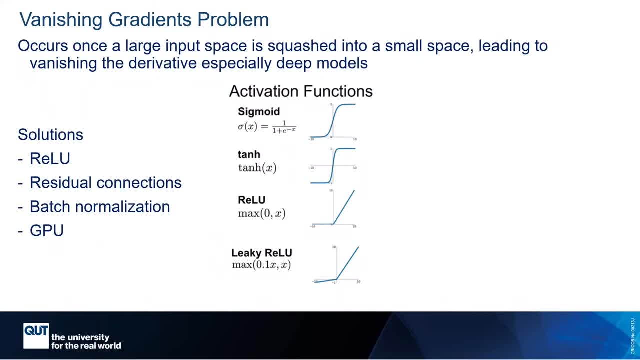 linear unit and liquid unit. There are other types of activation, So the problem of that means that the gradient will vanish by time of learning by just passing from layer to the layer. The problem is with sigmoid and tan-edge. these two layers just secrete the weights from one. 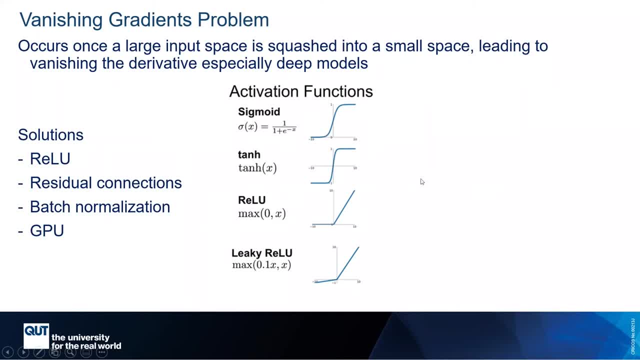 to minus 1,, 0, and 1.. So the problem will not occur when you have a shallow model, like few layers, because there is no way to squeeze. However, when you go with the deep models, these activation functions will keep squeezing the gradient until it finishes. There is no 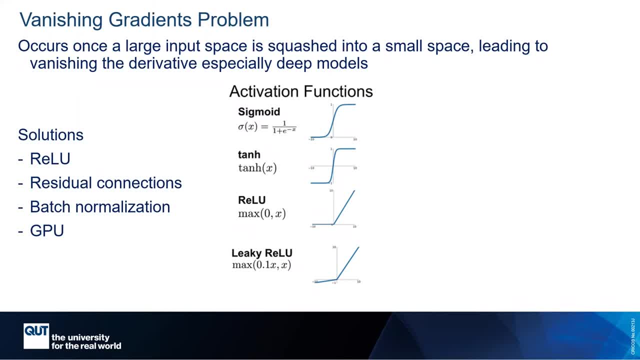 learning at all. You will get like zero learning after a few layers. In order to deal with that, rectified linear won't solve the problem by just taking from 0 to infinity and leaky also taking from minus 1.. So it will help in terms of avoiding the 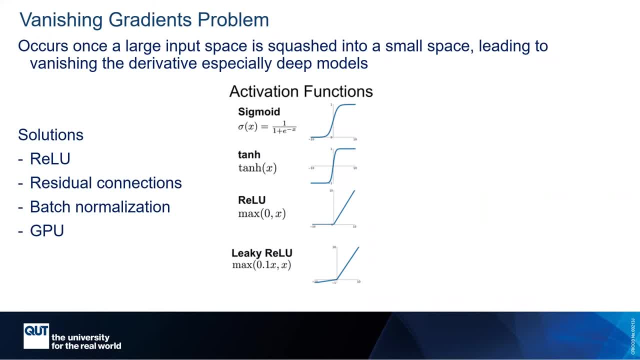 vanishing problem. So we're all aware of the good techniques and most of the recent models have been used to solve this problem. So we're all aware of the good techniques. most of the recent models have been used to solve this problem, So we're all aware of the good techniques. 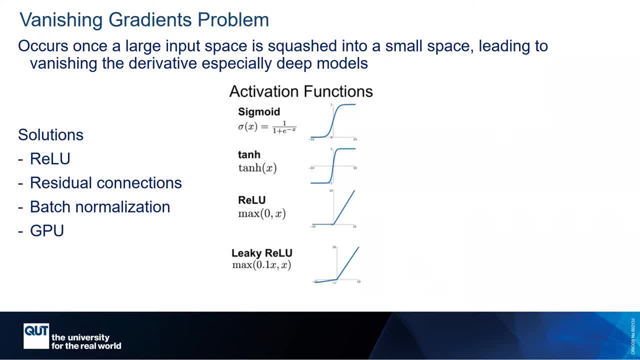 um, and these models use rectified linear to deal with that. Again, there is a downside of Roa which requires high computational tools in order to train them. However, with sigma and tatan age, it's not that high- computational to deal with these two activation functions. 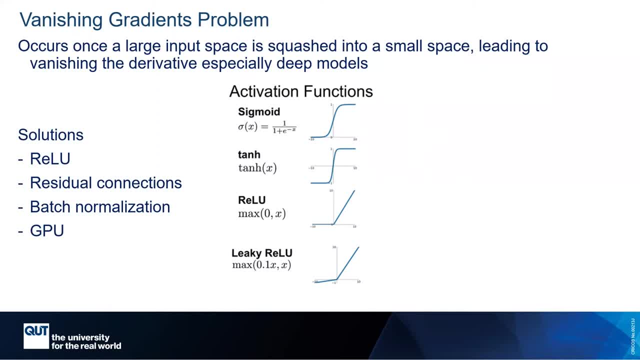 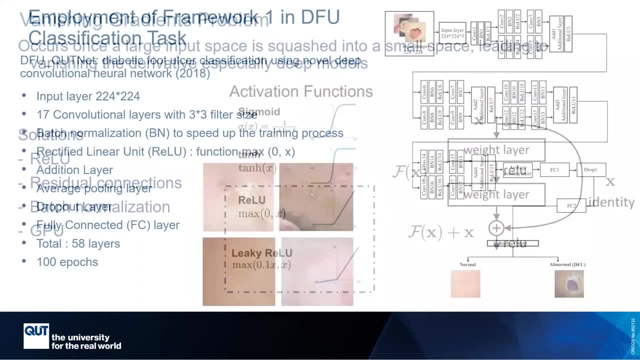 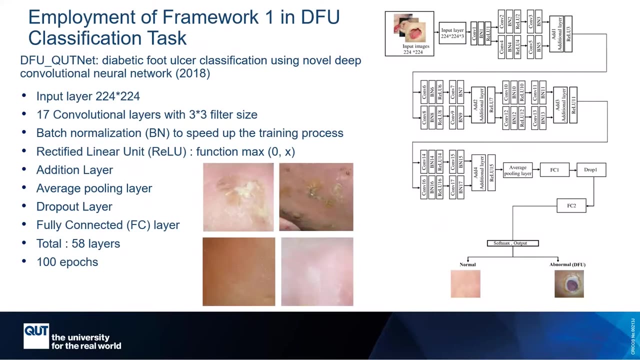 But again, it's based on the task, on the depth of the model that she use. One of the applications that we worked on- like around 2018, is we designed that model based on what we mentioned and on task of DfU- Diabetic Foot Ulcer. 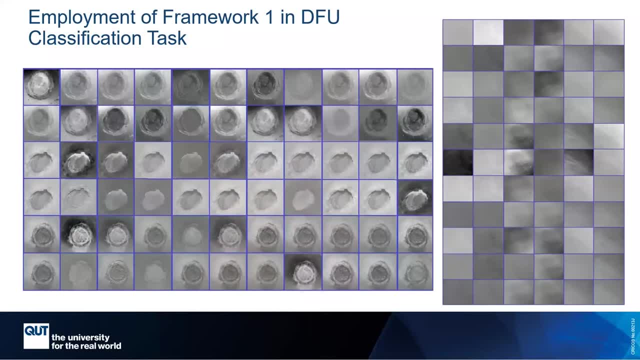 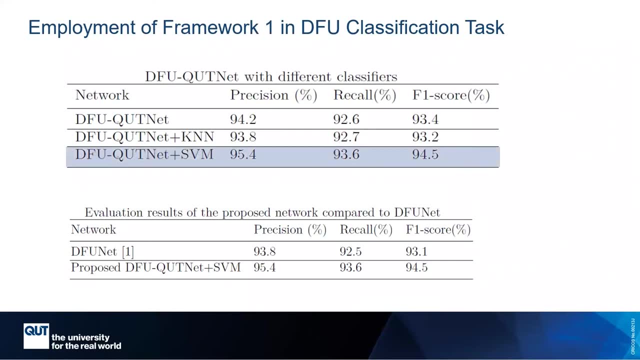 These are some of the features that we extracted and show how good to extract the features from the first layer, first convolutional layer, And we got the results that is really good: 9 to 5 precision and 9 to 4 F-scope. 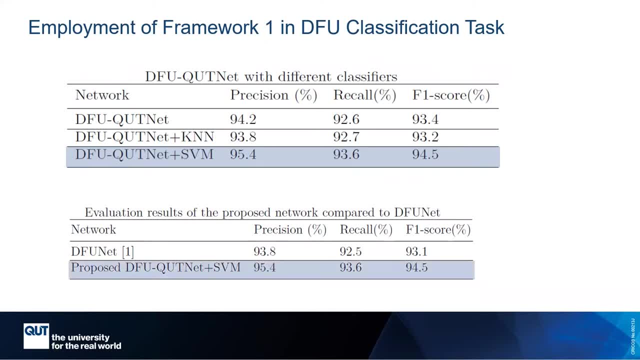 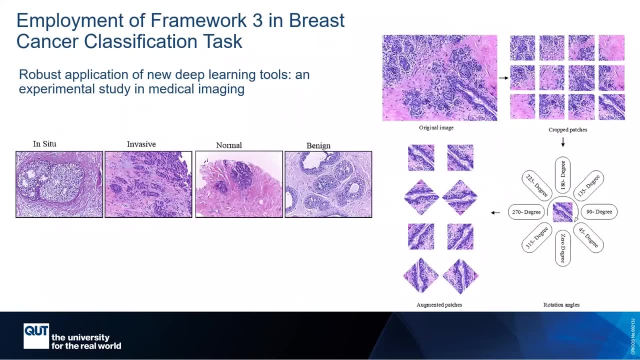 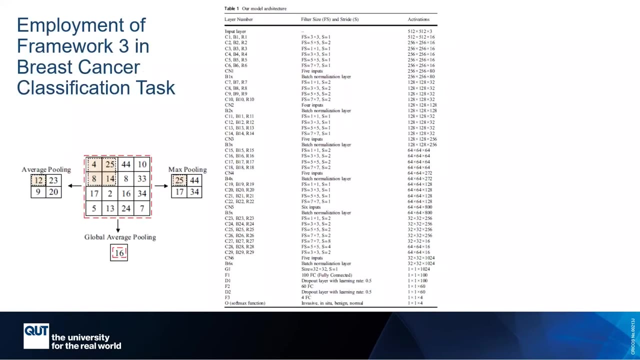 And we compared at that time with the state-of-the-art and we got better than the state-of-the-art. We did the same structure that we just talked about- the power convolution, the type of activation, function and different solutions with the breast cancer- and we used this type. 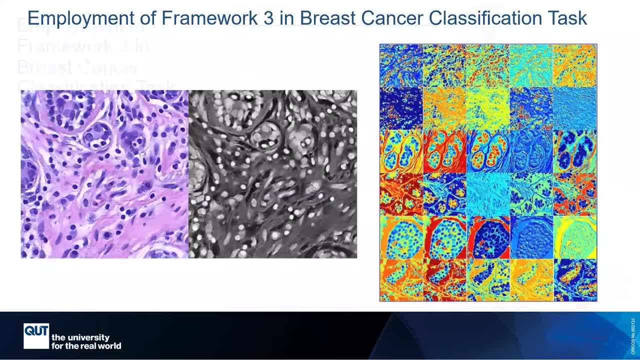 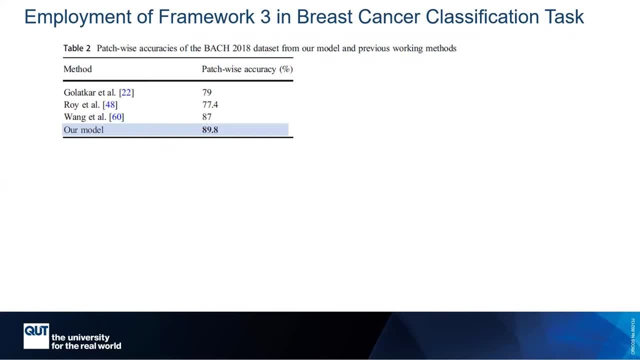 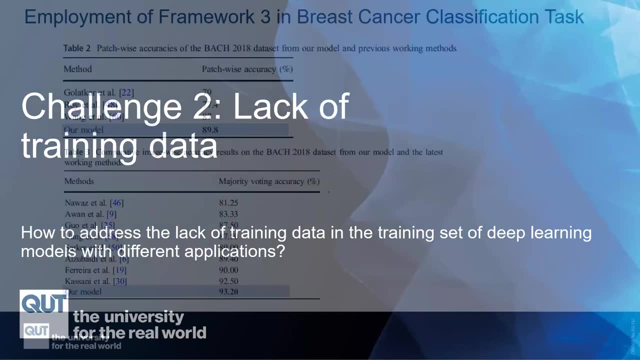 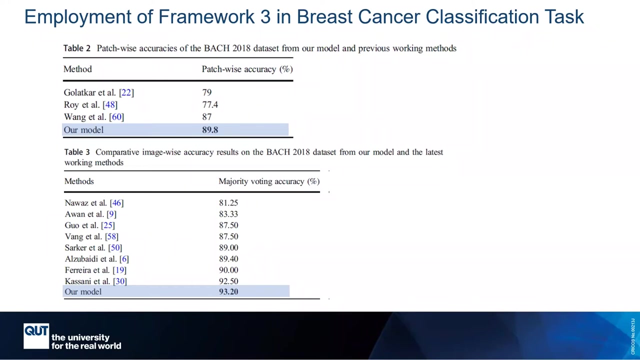 of models at that time And These are type of features that the model just extracted and showing how good in feature extraction And we got again good results on 9 to 3 compared to the all previous results at that time, However, still not that high, like 9 to 3 is good, but still the training data is small. 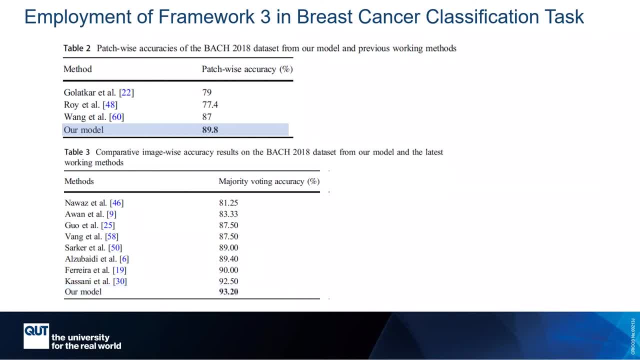 to train that very deep models. So in order to have good performance, You need to deal with data as well. So these are the problem of the structure of the design. by themselves are not enough to deal with the problem. So, in order to have a full image or full kind of workflow, in order to improve the performance, 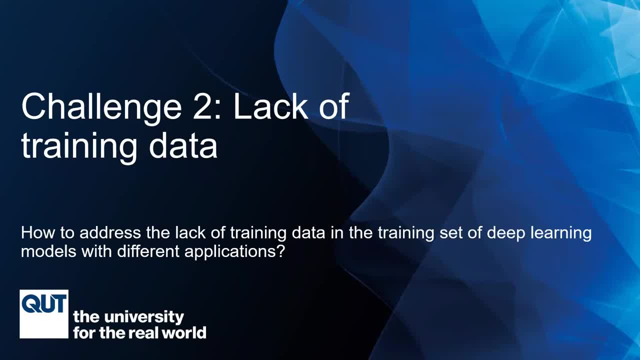 we need to work on both of them: the training data and the structure as well. That leads us to the second research question: how to address lack of training data. This is the most annoying question. The most annoying one is to have the data set. 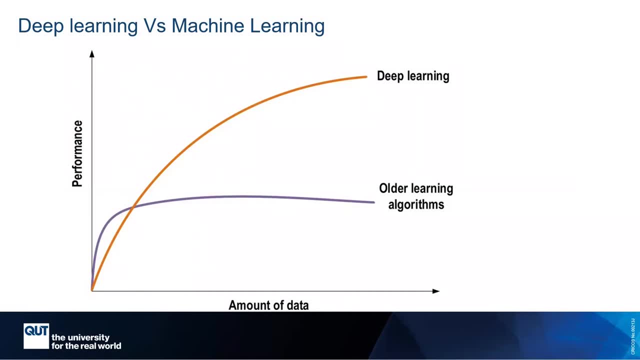 The good thing about deep learning: more data to give more improvement in performance compared to the old learning algorithms that they get to the point of saturation. There is no improvement in terms of learning even when you increase the data set. However, more data to feed the deep learning, more is good. 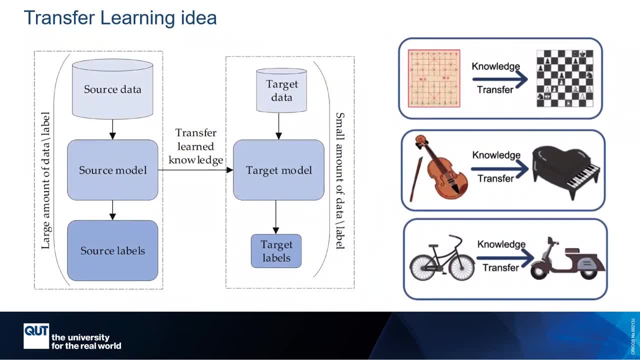 So it's hard to collect more data sets with the measurement Right. So when we think about the approach, if we look at data for individual, let's say for small data sets, for those when you have a large high based unit, for small data. 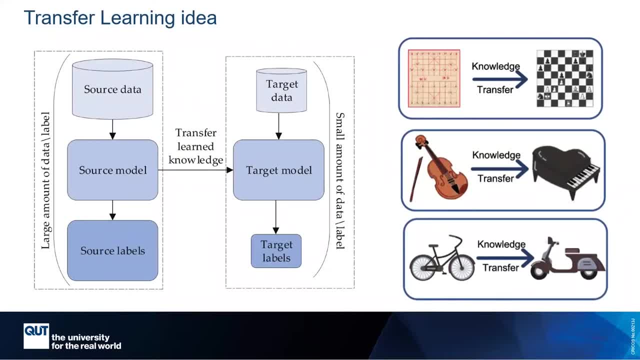 sets. you can't get more data set even if you have very small data sets. Or you can't get more data set even if you have a large area. then you can let the data flow by itself, right, Right. However, with medical image, you need to people who are really good and expert in the area and others to label that image. 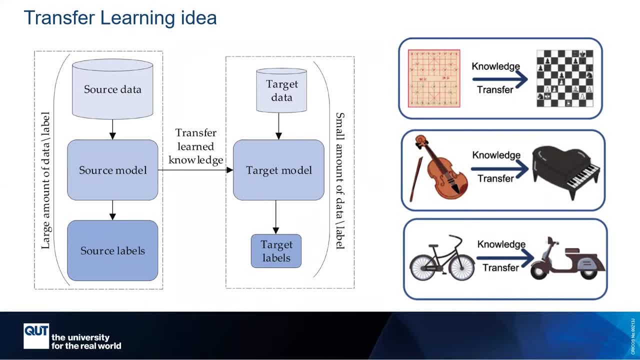 So one of the good techniques to deal with that is something called transfer learning. So transfer learning is a similar way of: for example, you know how to play violin. You just take that experience and movement and you hope that experience to work on piano, for example. 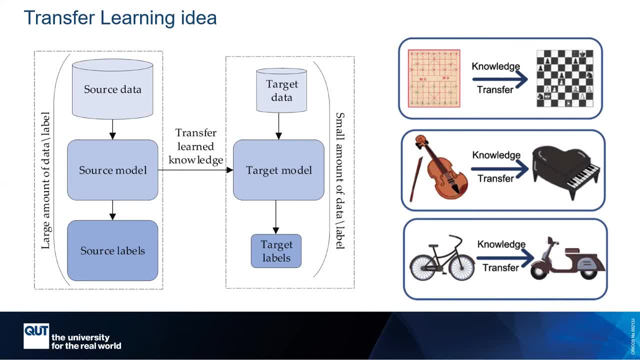 So imagine you drive a small car. you know how to drive the small car. you need to move to the big car, to the truck. You know how to drive, you train yourself a little bit, then you go to drive the big car. 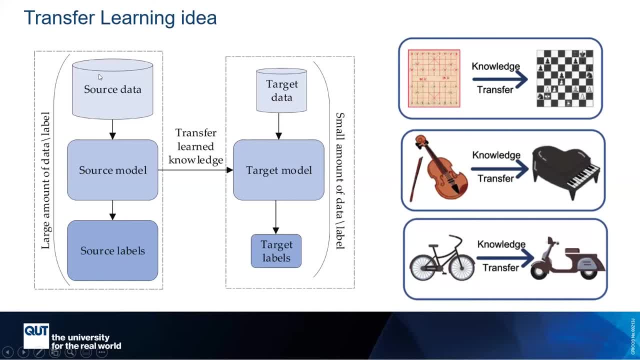 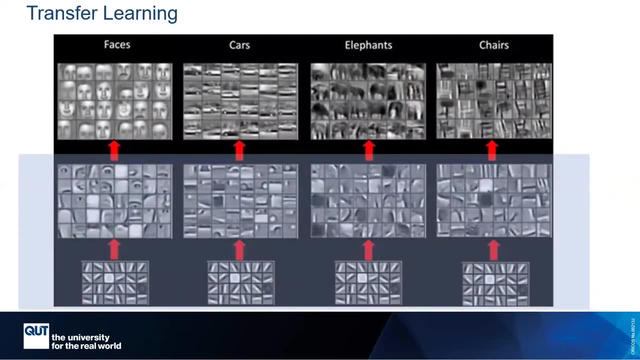 So the same thing here: like by learning from large data set, you transfer the learning to small data set. So this learning will help you in that small data set. So that's based on, they say, like the first learning On second levels of layers we'll learn just the features. 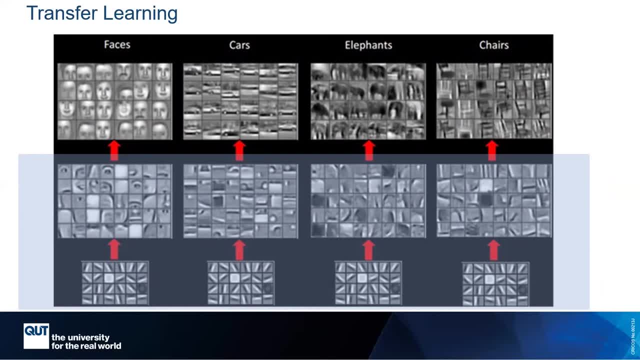 So it could be from any sorts of images. So that will help. But however the last level, we'll learn the specific features. So if I teach the first layers from similar images, then definitely then the small data set I have, I can just train the model to learn for the specific object. 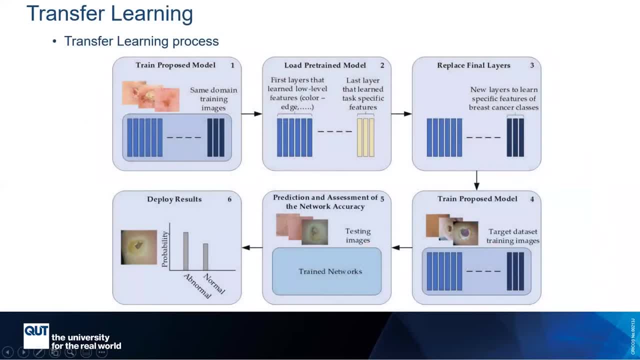 I don't need to go through all of that. So this kind of workflow of transfer learning: We're learning on the task, we move it to the last layer, adding the new layer to train on target data set and then train the model and deploy it. 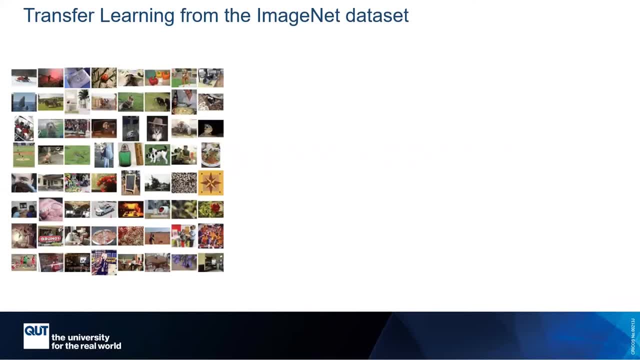 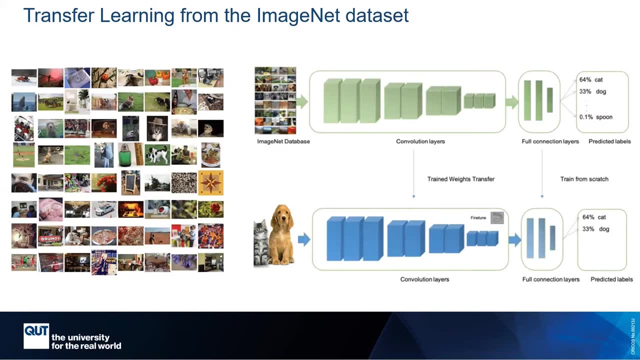 So one of the good techniques, of one of the types of transfer learning is to transfer from ImageNet the data set that we mentioned at the beginning. So several papers use that technique to transfer the features from ImageNet of these models like ResNet, GoogleNet. 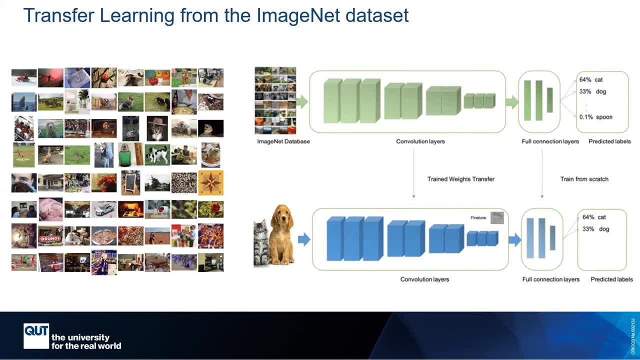 all these type of models and libraries to transfer from this data set to target data set. So imagine this scenario where we have a task to classify cat first dog. So there is a similar features between these, this task and this data set- And then, by doing that, the model already learned some of the features from that data set and then moved to train on the target data set and the classification. 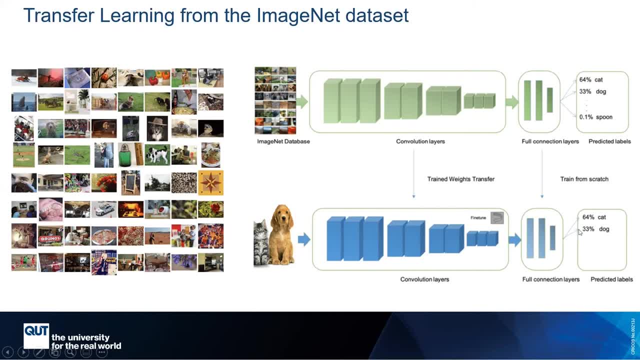 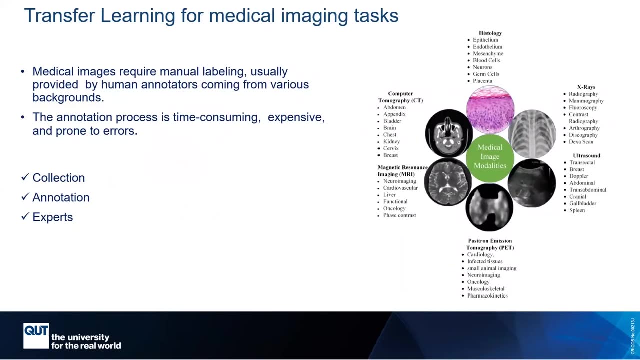 Which showed a huge performance, A huge improvement in performance in order to deal with a lack of training data. So with midi-color images- again we mentioned that this- these midi-color images require special pill, like collection annotation expert, In order to deal with that. 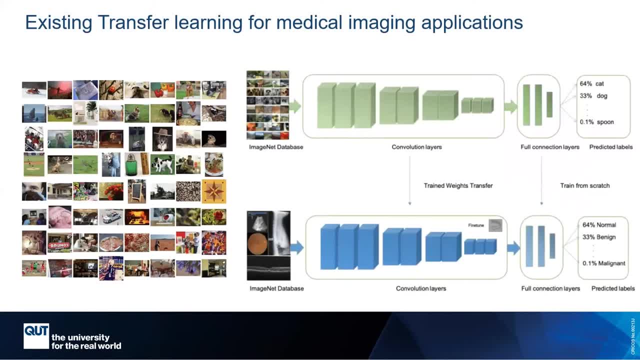 So starting people to use the same concept for midi-color images, Like using ImageNet in order to pull the performance of the mice, is very, very, very, very difficult to improve the performance of medical images and deal with the lack of training data. 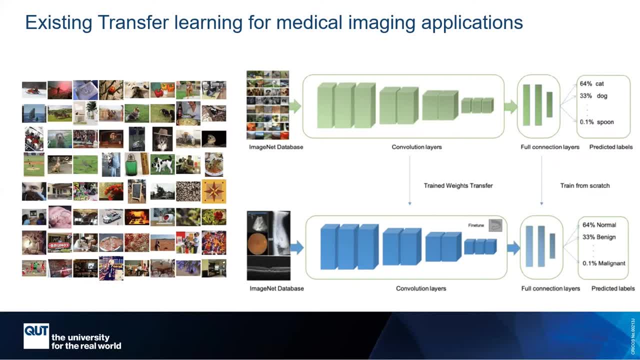 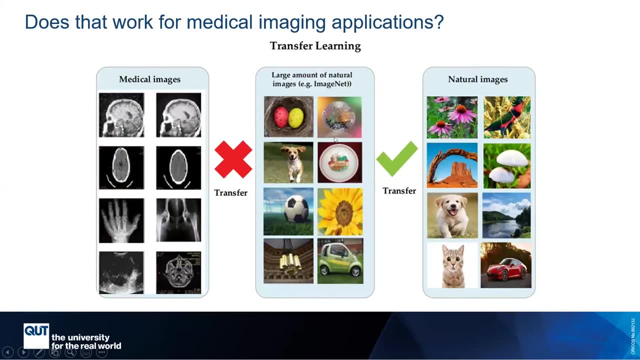 So that can help a little bit. until for specific task, However, imagine this scenario where we have this image net in the middle. you can transfer to the similar images with the nature like natural images. There is a common features between these, However, with medical images. 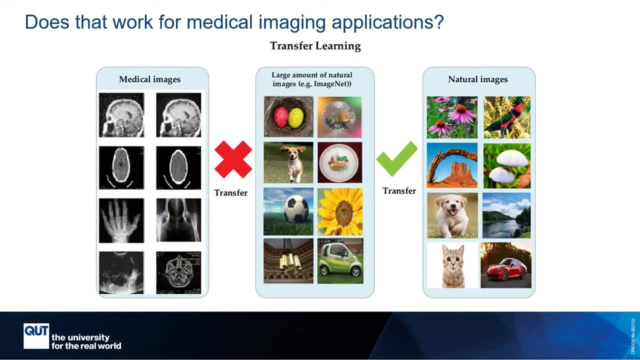 there is no any common or relevant features between two of these Several papers starting to investigate that the benefit of image net for medical images and they come up with a solution or with a conclusion that cannot help, especially for gray scale medical images. 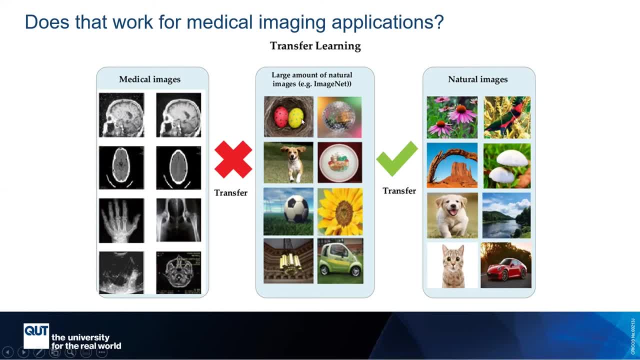 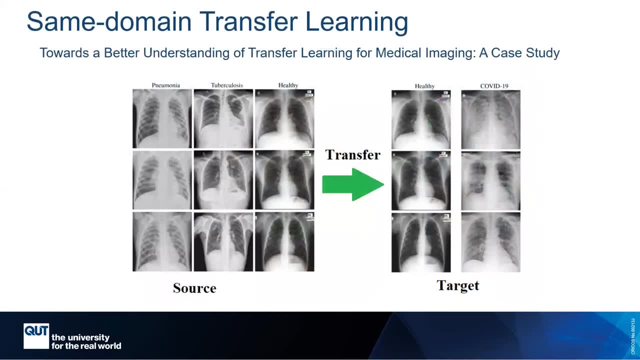 So these features are gray scale features. These are color features. There is no way to learn from them or to help them How to solve the problem. As a part of my PhD, I did an investigation on that. I've come up with a conclusion. 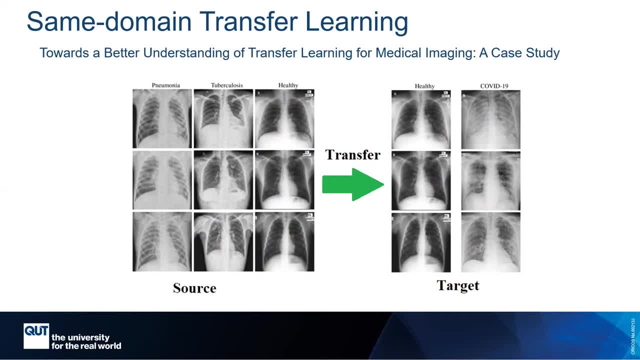 that these models cannot help. So I come up with the first type of transfer learning. In order to do a transfer learning from image net, you can use your own transfer learning. So imagine the scenario where we have a healthy-owned COVID. So there is no large data and like a number. 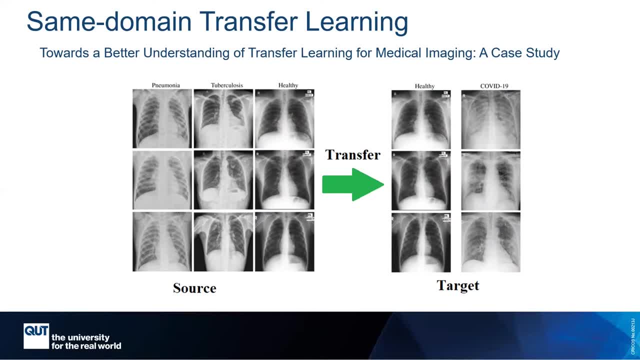 of data set. when COVID started to like around. scenario there is 200 by 200 cases for each class. there is no way to train the deep learning with a small amount of data set. even if you get high performance, definitely the model is experiencing overfitting if you move on to the different data set for covered- unhealthy definitely you will. 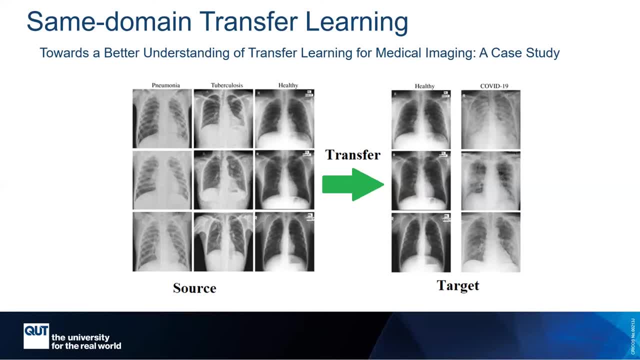 face the overfitting problem. so what we did, we, we, we started by training the model on same domain, transfer learning with the same environment. so we have a large data set of pneumonia, different type of x-ray, like a huge number of x-ray, like around 250 000 images of a chest x-ray. we first trained 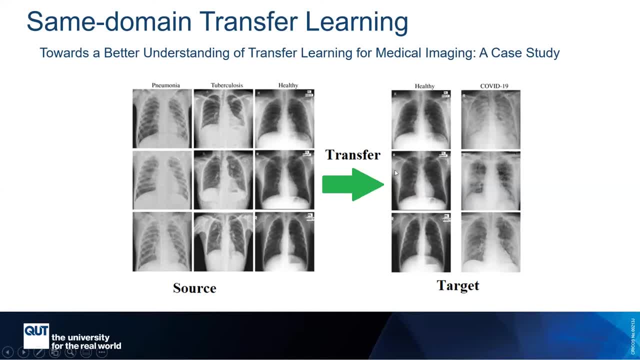 the model on that. then we did the transfer learning on the target data set. we compared between from scratch training on the target data set with the proposed transfer learning and we came up with the conclusion and with the results that showed a huge improvement in terms of performance and generalization by testing on different data sets. later on we found that the 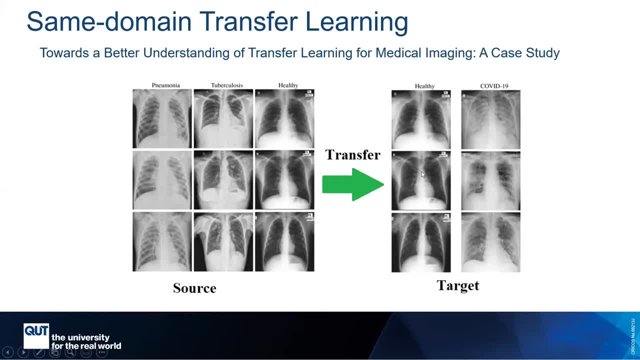 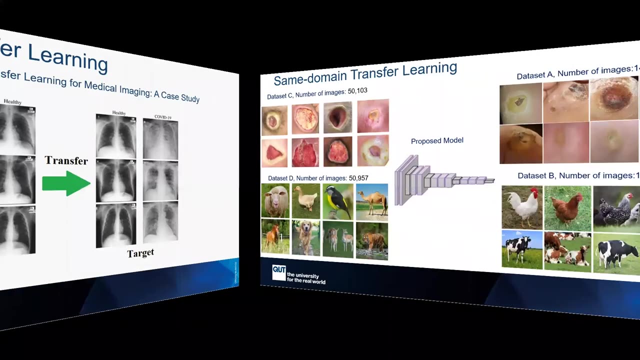 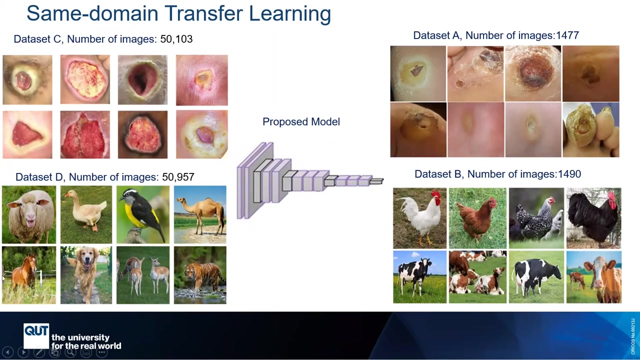 model of training from sikraj just showed bad results on different data sets. however, this one with the transfer learning showed good performance, good results when we tested on different data sets. not only that, we found out later on even with the color images, of medical images, if you choose. 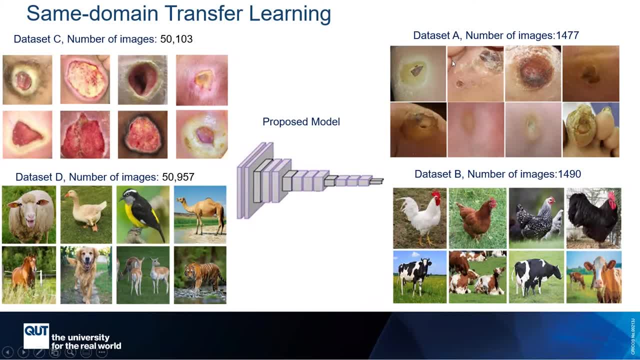 image net from environment to the medical data set, can affect the performance. however, if you use similar tasks, for example dfu with wanted, and then there is improvement in terms of results, even with the color images. so the source of a transfer learning is really important. so, for example, we 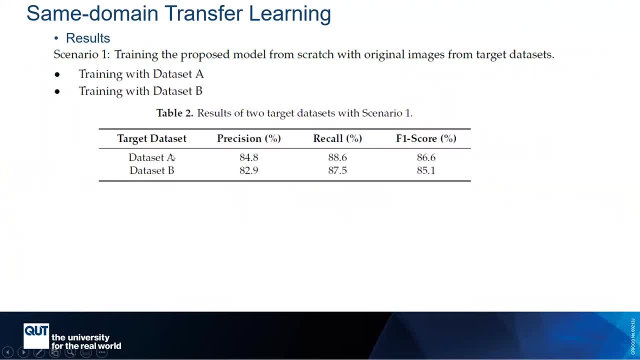 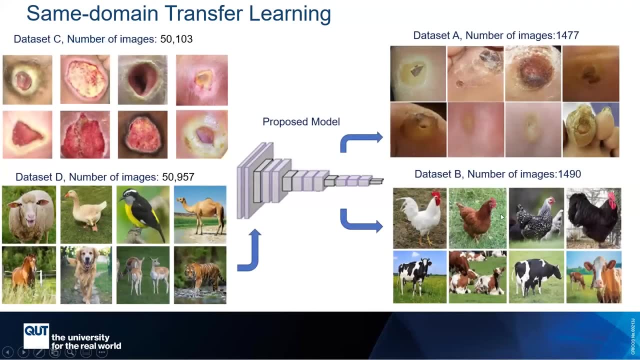 we use that um by transferring from image net, we got this result. i mean data set one and data set two. this one, data set one and data set two, is the source of this one from here or the source from here, and the same thing for that data set if the source from medical or from same domain. 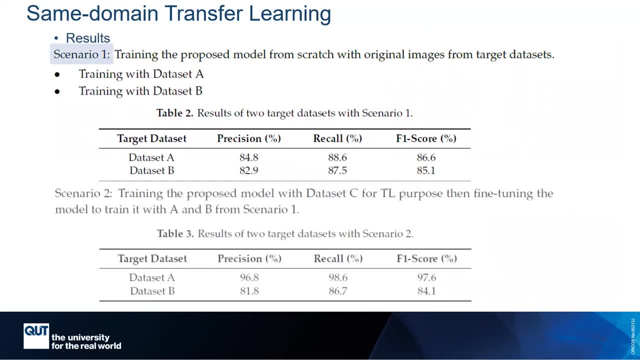 the purpose of the study to show that even with um, even with the color images, if you're taking the source of transfer, learning from same domain, it's better having like large amount of data from different domains and showing here, by just choosing the data set, a with the medical one. 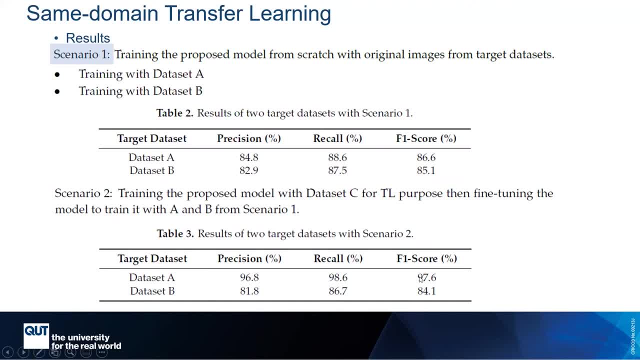 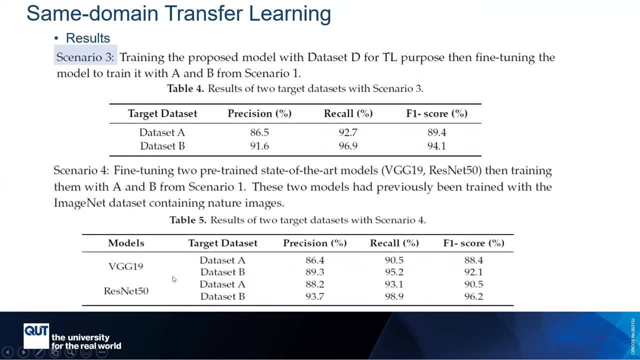 from the source of medical uh transfer learning got 97 percent. however, it got already um scenario where we train from the image net. so that showed that uh again, even with. compared to two models- vgg 19 at that time and resnet- and both these models showed uh less performance. 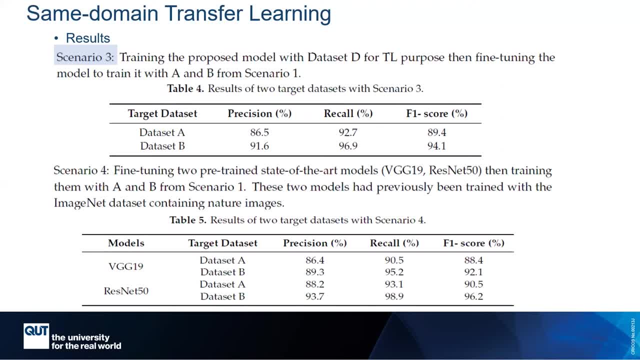 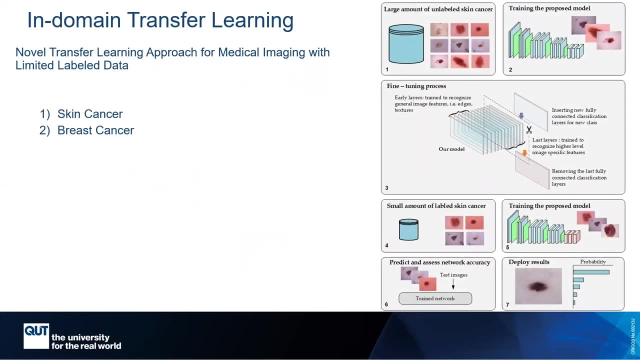 which both of them trained on 14 million images, less performance than the model that we proposed by training on the source, that similar date, a similar domain. another way of transfer learning did with the skin cancer by just collecting a labeled skin cancer, because the purpose of transfer 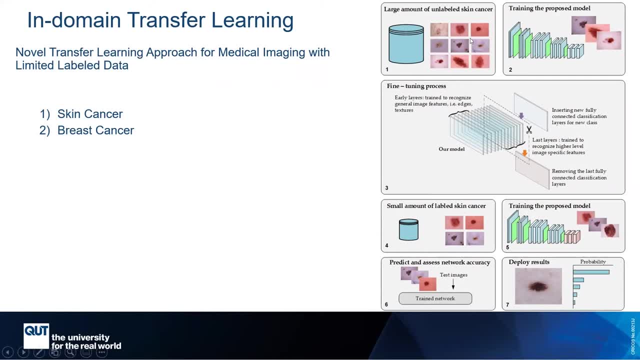 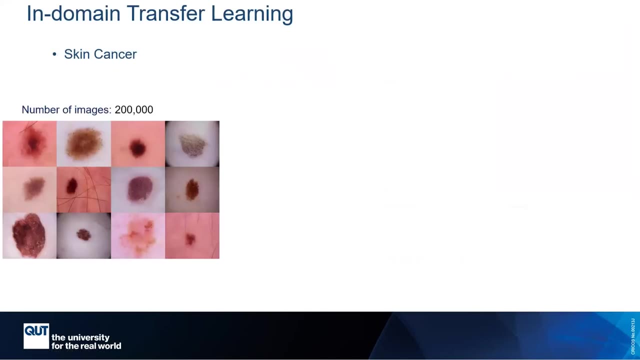 learning is just to get the features. then we collect a large amount of unlabeled skin cancer. we're trying the model we did fine tuning. then we're turning on the target data set and then after that we compare that results. so we did that by collecting 20 hundred thousand images of skin. 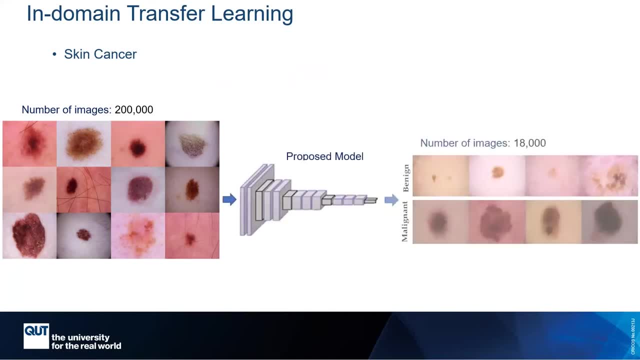 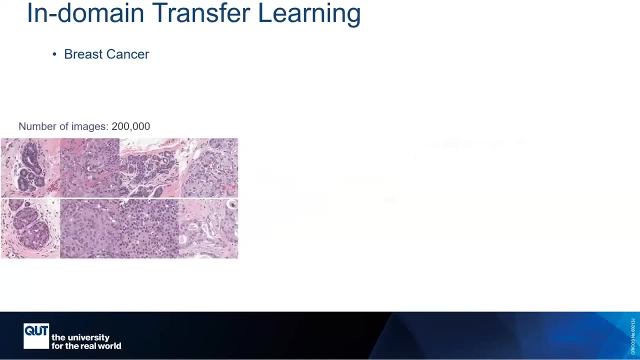 cancer a label. you don't need to label them. then after that we fine tuned that model on 18 000 images of skin cancer. we did the same procedure, with less amount of training data, with breast cancer also, the source was histopology images- 200 000 images. these are some of the. 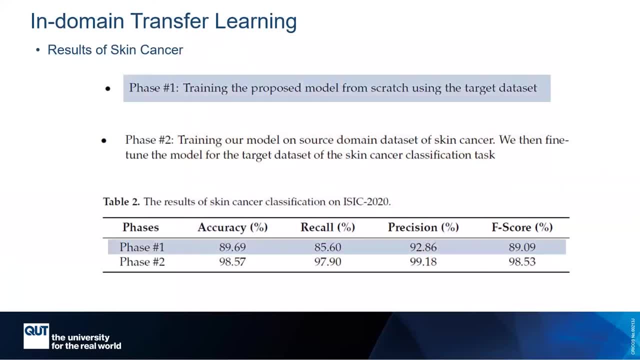 features that the model extract. um shown here that when we use the target data set like with from sikraj 989. however, with the proposed transfer learning we got 98 percent accuracy fscore by using the proposed transfer learning um. later on we tested both models that. 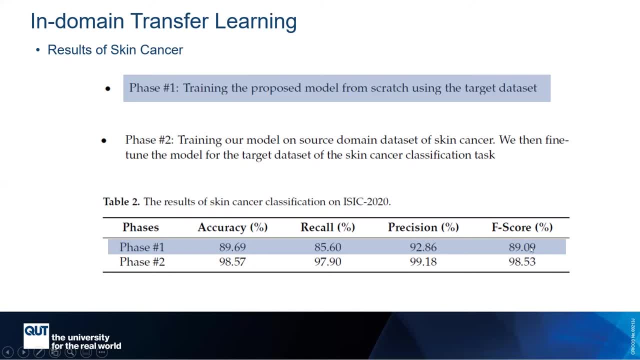 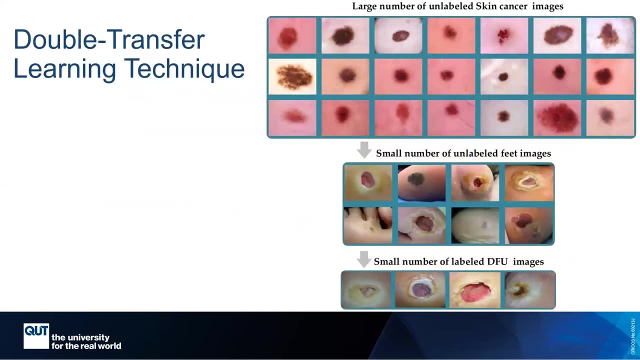 trained from sikraj. that model, when tested on different data sets, got bad results because, even with the 89 percent, still not generalized very well. however, the 98 percent got really good performance on nc data set. not only that, we use the same model that trained on breast cancer for. 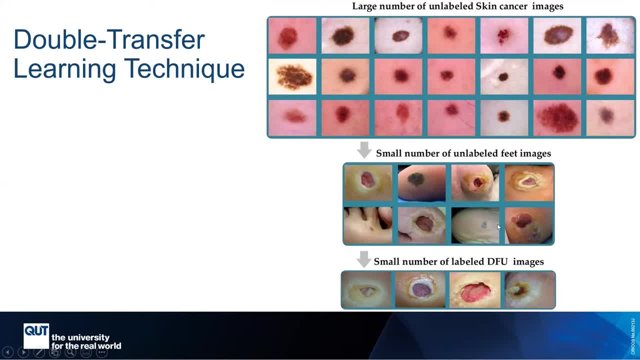 different tasks by also creating a model that trained on breast cancer for different tasks by also collecting similar for the diabetic food also. we call double transfer learning on that breast skin cancer model. we fine tuned that model on unlabeled fit images then for the target data set. 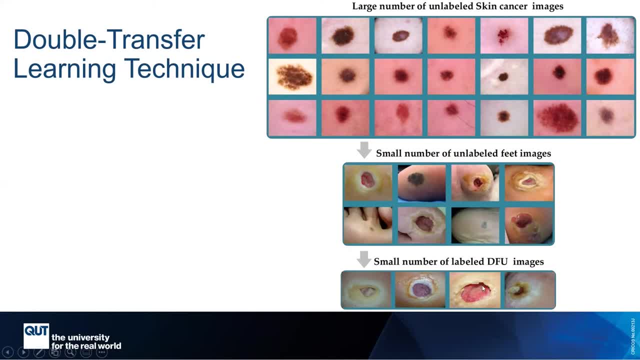 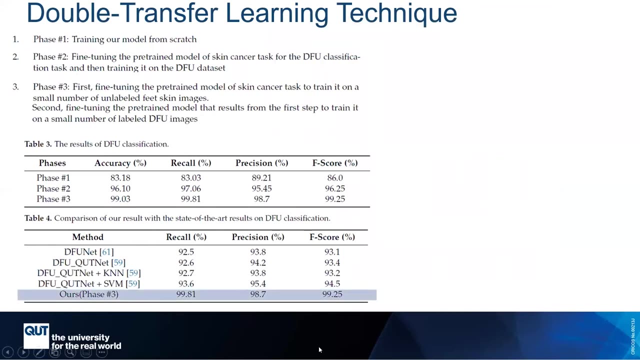 so, in order to improve the, the features a little bit and then on the small amount of labeled, the purpose is to reduce the need of label and then and then will reduce the need of uh expert to spend long time again. the, the third uh that proposed uh, showed 99 percent and generalized very well by showing that these 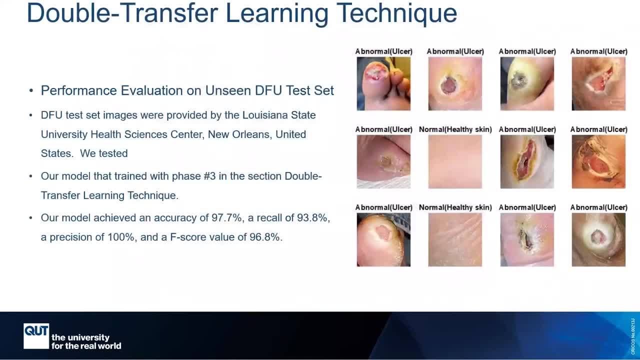 are the features that the model extracted from the first layer- and this is an example that i kept this example in order to show later on that model tested on nc dfu data set from different environments, from different countries. we um the data set were provided by louisiana state. 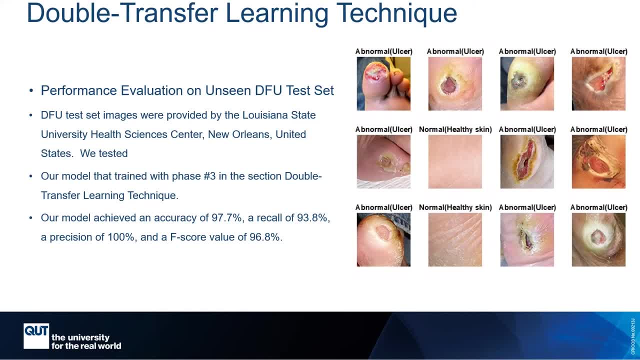 university of health science and we got without framing on that that they said just for testing. we got 97 um accuracy, 93 uh precision and 100, uh sorry- accuracy of 97, recall of 93, position of 100 and score of a score of 96, which showed really good performance on nc and this way that showed that. 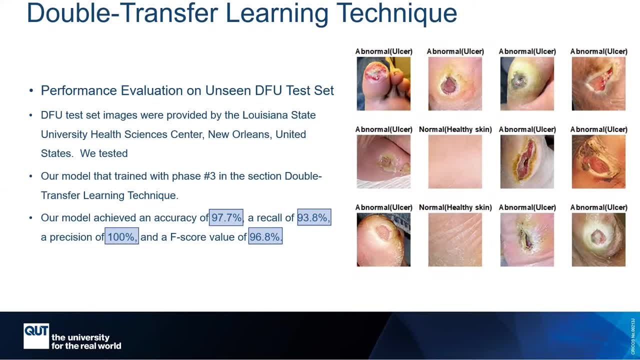 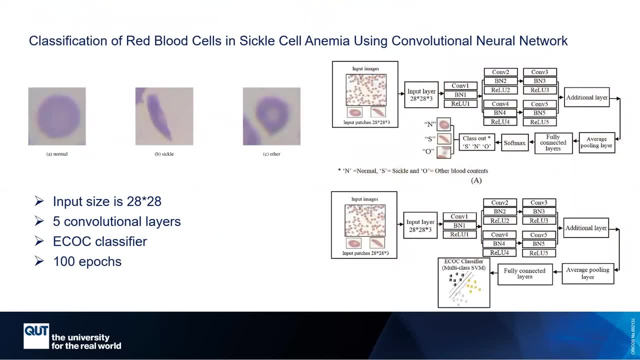 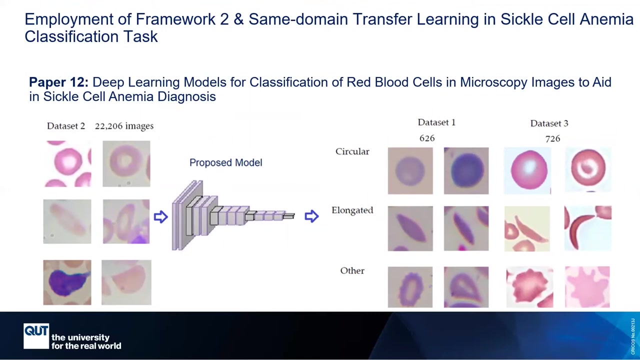 the model generalized, very well able, not even not experiencing any overfitting. We tested that concept of transfer learning, several types of transfer learning, on different tasks. We tested on red blood cells to detect sickle cells anemia. We did the same thing. We got the same source domain from white blood cells to the red blood. 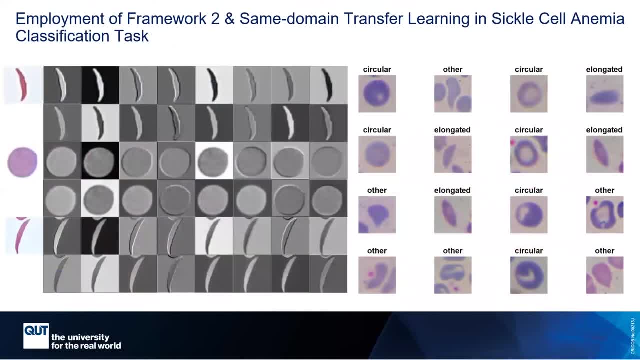 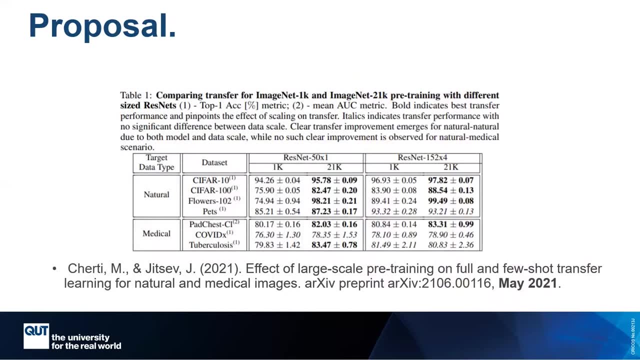 cells. We tested that on different data sets. We extract the features and the prediction. Later on, several papers started to do the same thing And, for example, this paper just improved The source of transfer. learning is important to be in the domain and showing that if you take the 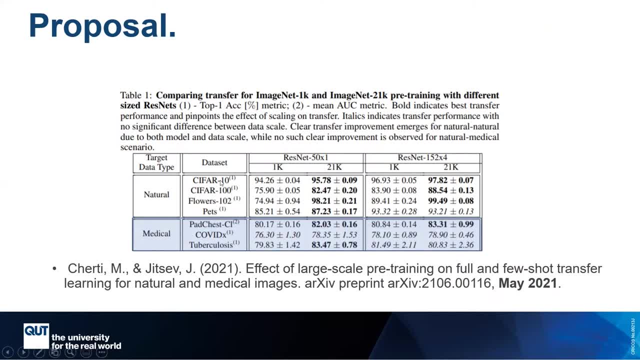 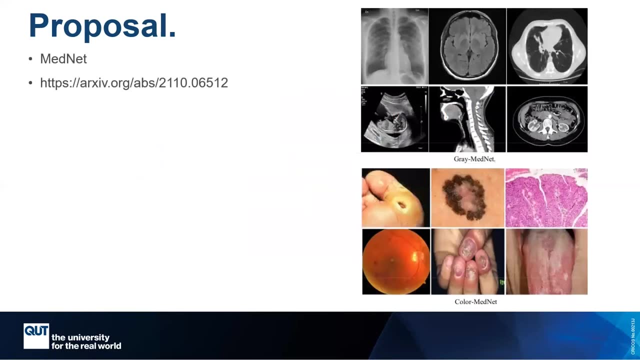 natural images from these natural data sets and do the transfer learning from Imagenet, there is improvement in performance. However, if you use the Grace government, for example, COVID, there is a drop in performance compared to these data sets. So it's important to have a source of transfer learning. Later on, I proposed a model called 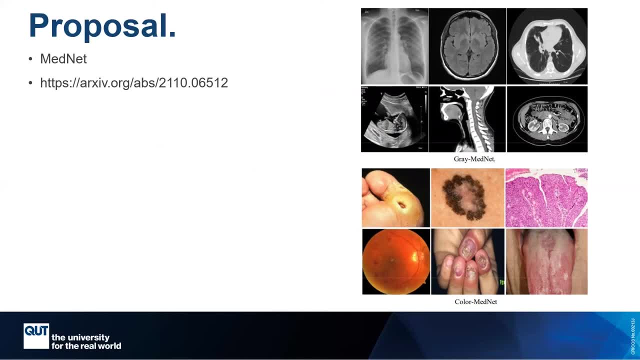 MitNet, which I aim to have, a model that will train on a huge amount of data, of grayscale data. Then the researchers, the community, will start to fine-tune that model for their task. There is no need to train on large data sets. However, I haven't implemented, just proposed something due to 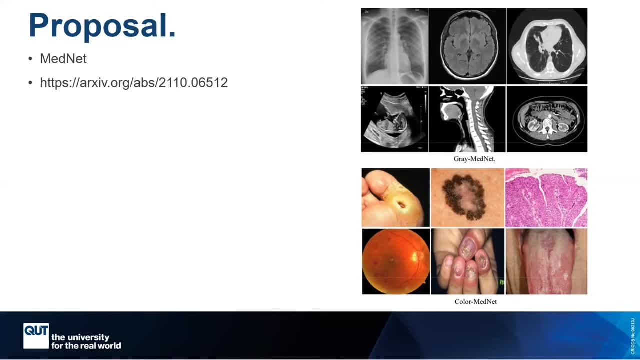 the high computational tools. I'm aiming to train that model on 3 million images publicly available and the same thing with two versions and the color one. Then that will help a similar way of Imagenet to have a model that trains on a huge medical data set. From that time I proposed that 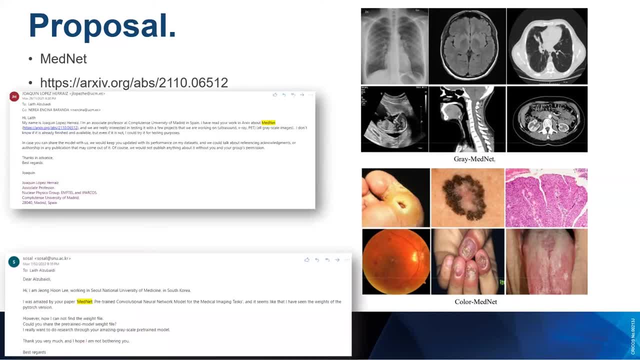 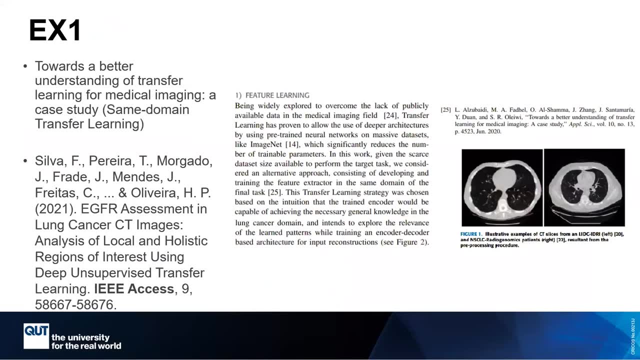 I'll publish it online as a proposal. I keep receiving emails asking for that, which I haven't implemented yet. The same concept that we propose by using the same domain or from large data set or double transfer learning stuff. Many papers just use the same technique for different tasks. 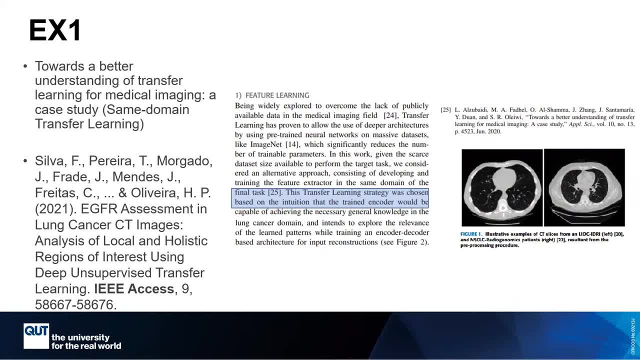 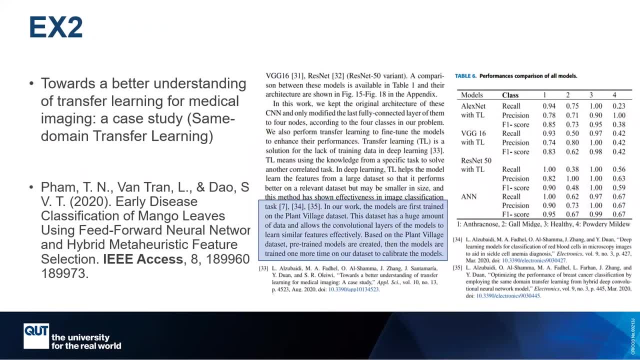 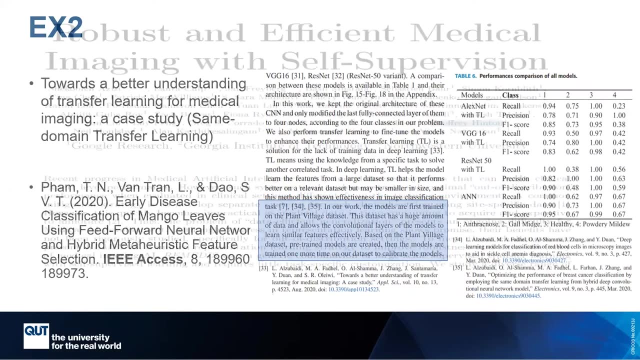 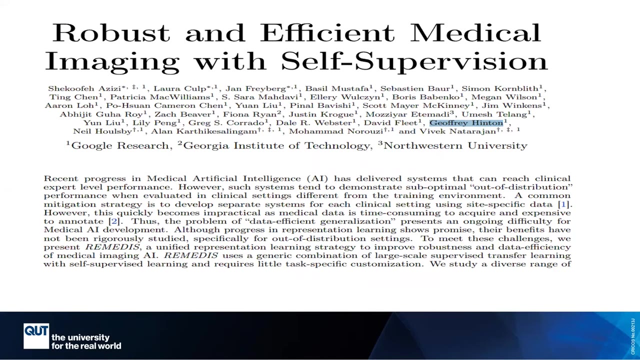 like CT and they showed a huge improvement in performance, significant improvement. And another paper: even they used for agriculture and they found out that it's better having same domain transfer learning than transfer from Imagenet. Lately, the founder of deep learning, Jeffrey Hinton, just released a paper with the 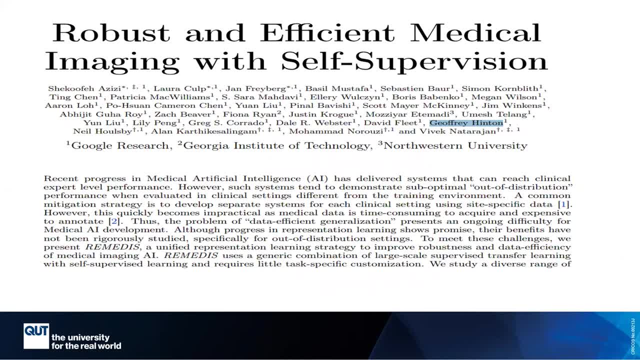 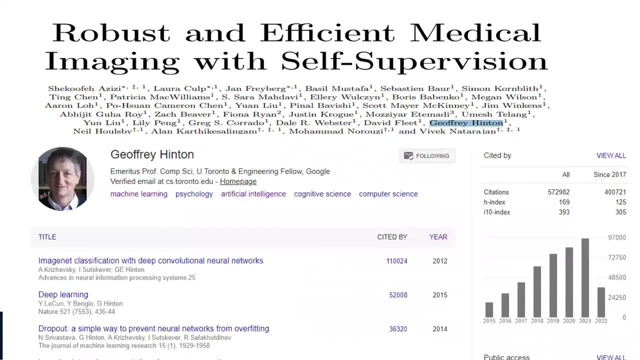 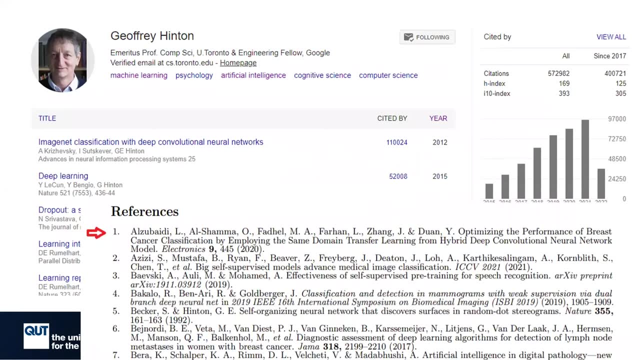 Google Research Group, showing that self-supervised, which is from the same domain, is better having the Imagenet for grayscale medical images. This guy is the founder of deep learning and the father of deep learning and even just pointed out to two of our 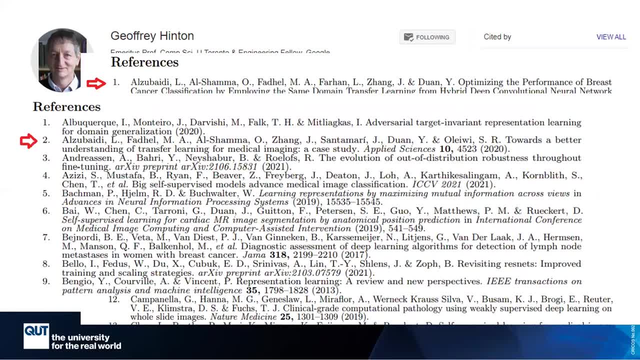 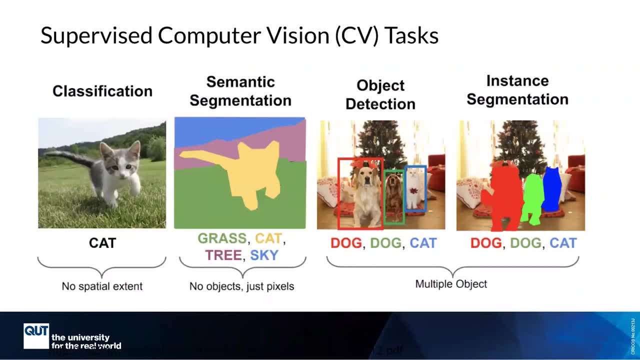 papers that Imagenet. this is type of transfer learning tools for deep learning. Transfer learning is able to deal with any type of these. You can just use transfer learning in classification or even segmentation, detection and so on. Once we learn the features, we are able to use them, Whether 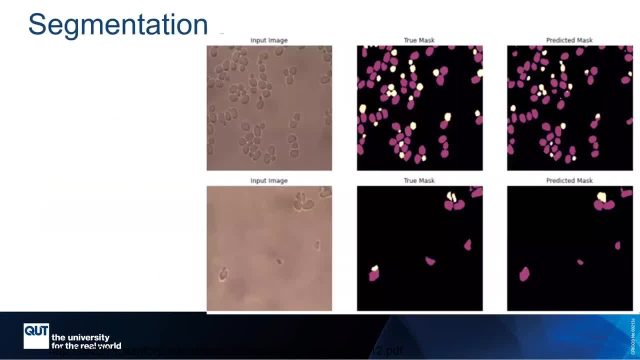 it's a classification or segmentation. any type of medical or any type of application can just implement the transfer learning, But the point is how to train on large or similar source of transfer learning. The point is nowadays, I believe, that moving from big data, 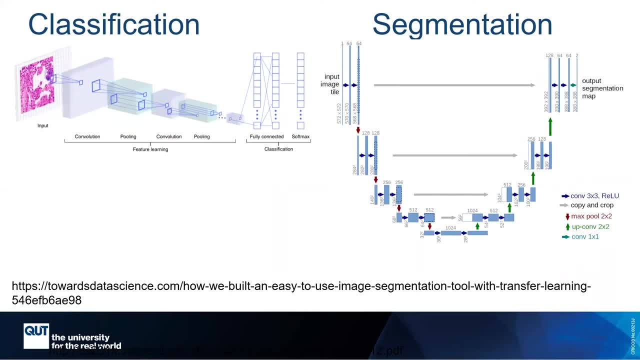 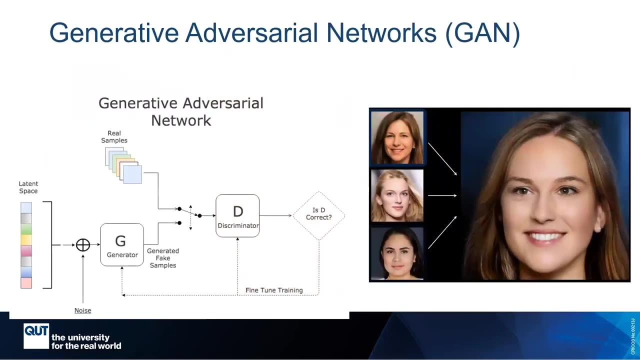 more big labeled data to this small amount of good data. like having small amount of training data, like small amount, then you can use definitely transfer learning in order to deal with that small amount of data. Another solution to deal with the lack of training data is Generative Advertisement Network. 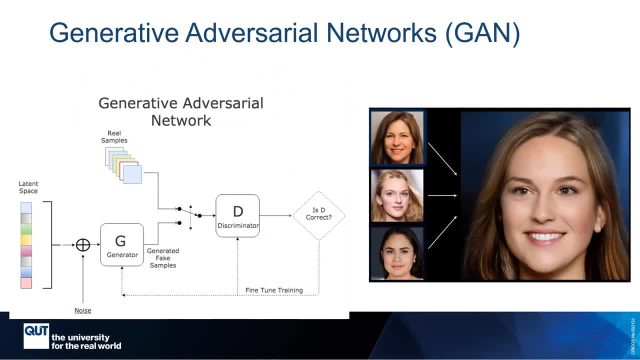 is GANs. There are several types of GAN purposes to use TASCAN. The simple way is basically to train from real samples and there is a discriminator to say whether it's real or not Or if it matches with the real samples. just return an input to come up with the new sample. 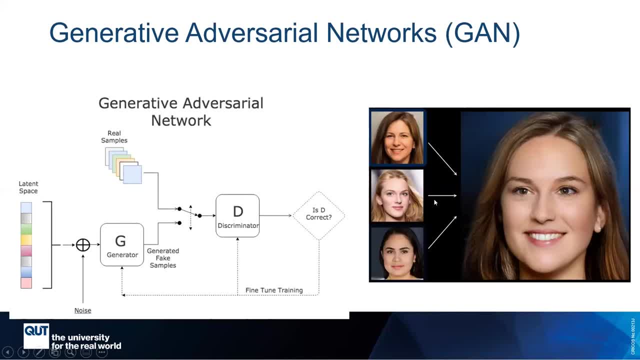 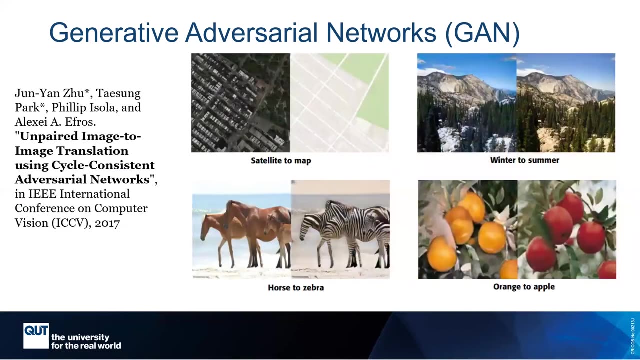 Let's imagine this scenario. We have the three input images. The network will get the features from them and build a new image that's not similar to these images. This kind of technique helps in terms of generating more data to train the deep learning models. Also, one of the types of GANs is 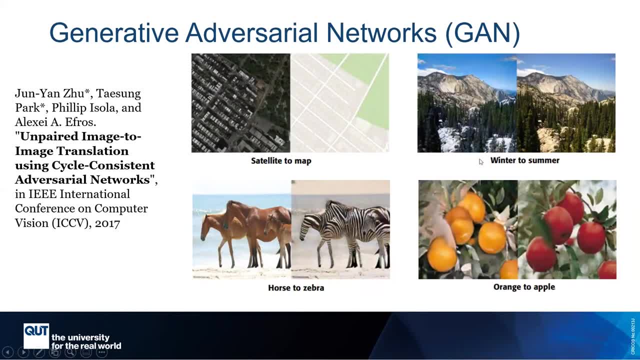 to convert, for example, from satellite to map. This is a good example of how to convert data to winter to summer, or horse to zebra, or orange to apple. Just an example to show how to modify from one sample to another. 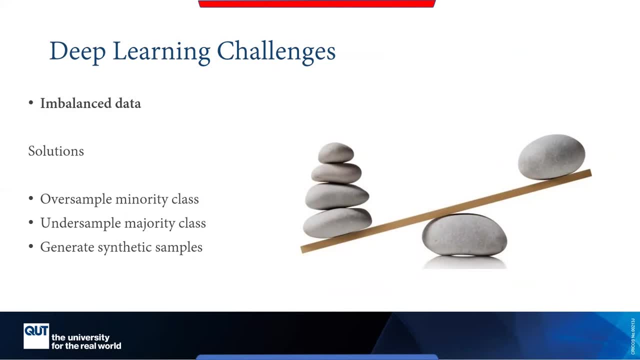 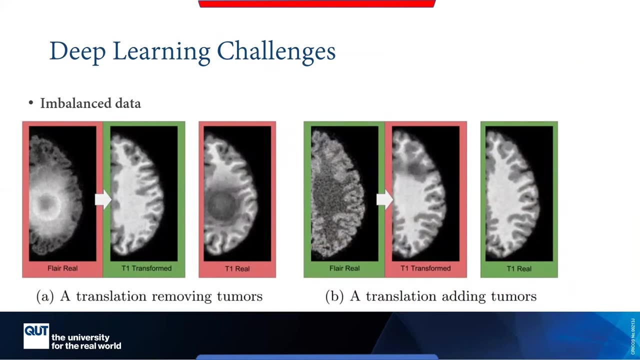 Also, GANs are used for unbalanced datasets, For example. imagine the scenario where we have high number of normal class and small number of abnormal class. I don't recommend that you train any deep learning model with unbalanced data. Definitely there is a problem. 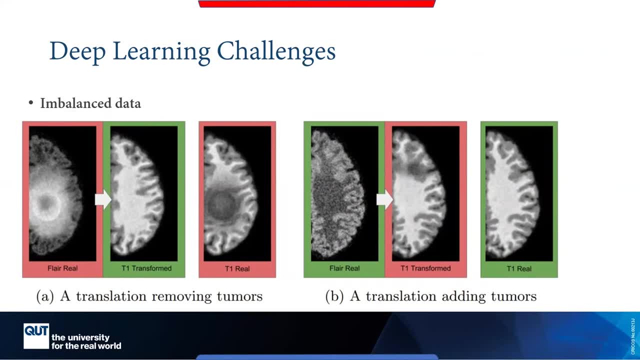 with that, unless you evaluated on different evaluation metrics than the accuracy and precision and the score. But you need to think of a way how to balance your data before you train any deep learning model, because the model definitely will overfit on one of these classes. 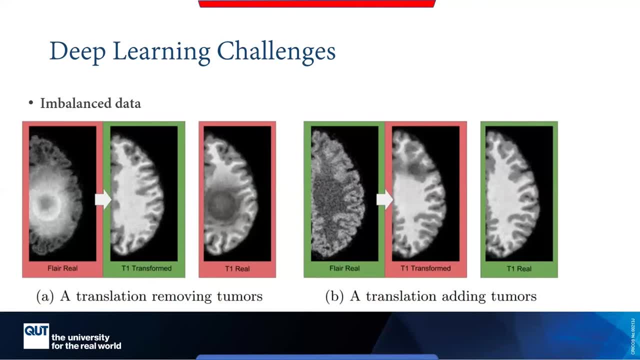 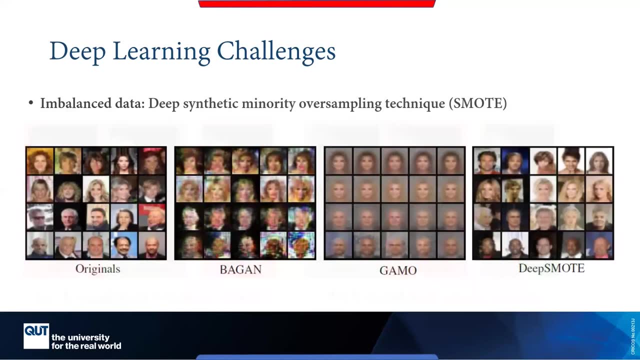 So GAN can just convert from, for example, normal to abnormal, Of Normal to Normal, to generate more samples. Another technique called SMOTE that helps also to generate more data. there are several algorithms and this one just released in 2022, comparing. 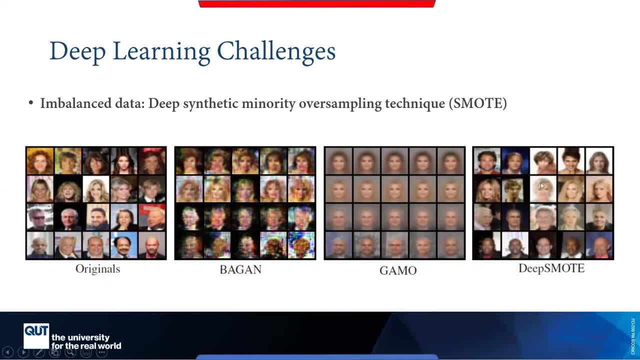 with GANs- different types of GANs- and that paper proposed that they are able to generate good images compared to the GANs from the existing images. So two different images that help generate more data. there are several algorithms and this one just focused on power circles. So, for example, these are a few algorithms that are justчеering the front end to the sides, not into the back end of the Landscape object. they are able to generate good images compared to the GANs. A lot of them are can be done by other combining, While in larger scales, just as that someone that 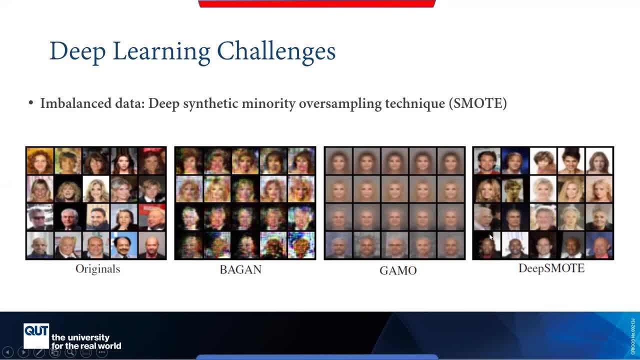 produced. the graph was running some measurements and they can use them in a normal approach. you can really see how powerful this analysis can be in the moving time. These are kind of сказ haruso to images. there is no need to high number. maybe 100 can generate another 100 of images. 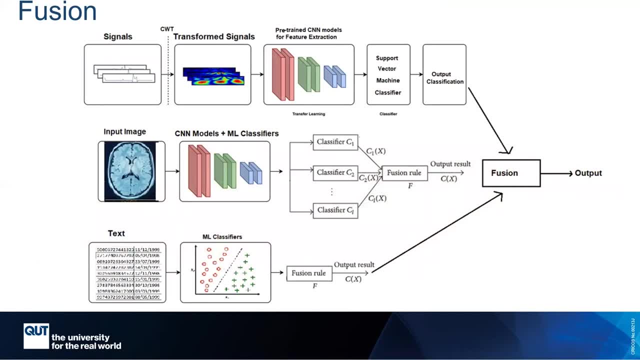 Last but not least, one of the good ideas for medical images, which I believe is fusion. Fusion is a good technique to give robust decision, For example, could be: same source can use several algorithms, then fuse them in the one decision or maybe the task that. 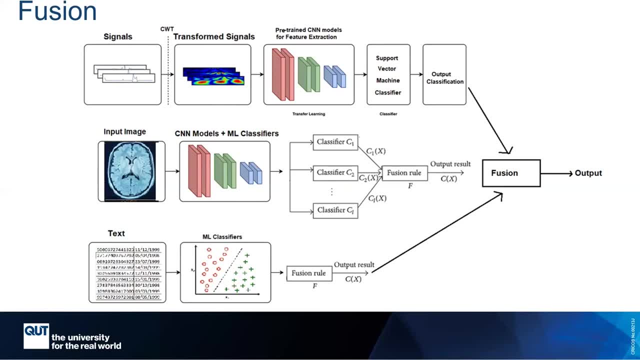 you have a different type of data, and then you can just basically do a fusion on that by, for example, work on signals, come up with a classification, or work on MRI and come up with the classification, and then text data, numerical data, whatever you have, and then 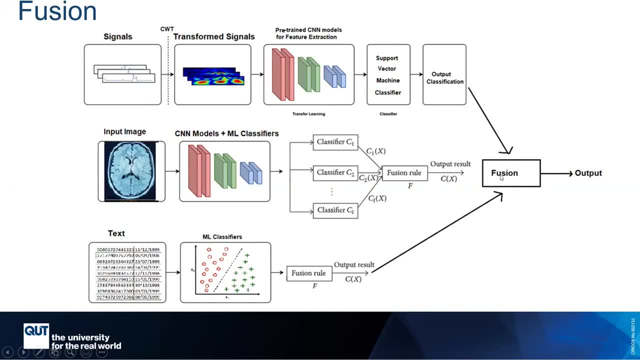 come up with the three decision and do fusion here, different ways of fusion, and come up with a final decision. So the decision. So based on different types of input for one task- or maybe you have an MRI- you can just use that input image with different algorithms and then fuse them in one final decision. 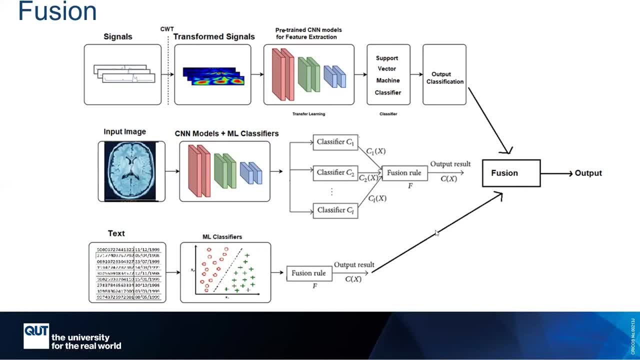 That's a good way to give robustness to the decision in order like one problem, that three opinion on the same problem is better having one opinion, in my opinion, or even you can just do something called waiting. If you always find this one is the most robust one, you can give like 90% of the decision. 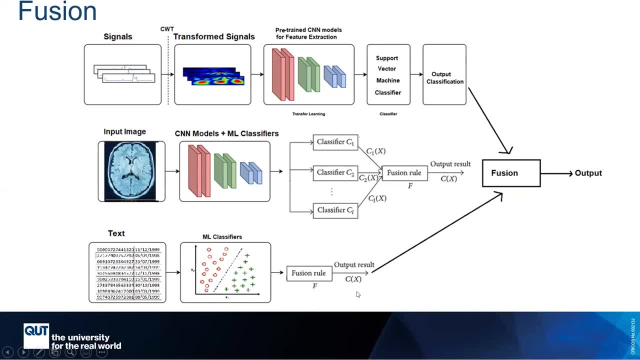 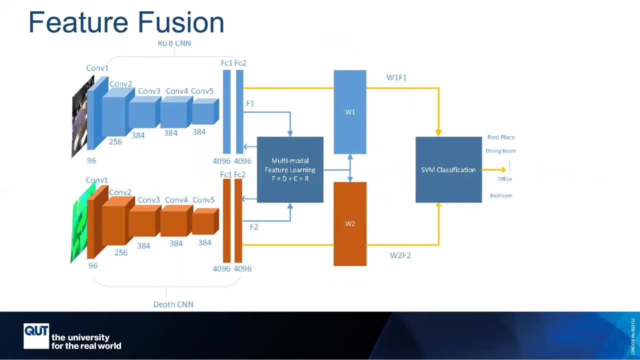 or 70% of the decision on one on 20%, which can reduce the error somehow. Another type of fusion called the future fusion. you use deep learning models, you fuse the features that extracted by these models and you feed it to the machine learning classifier. 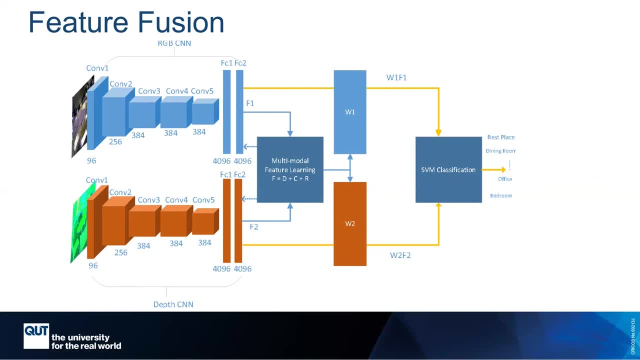 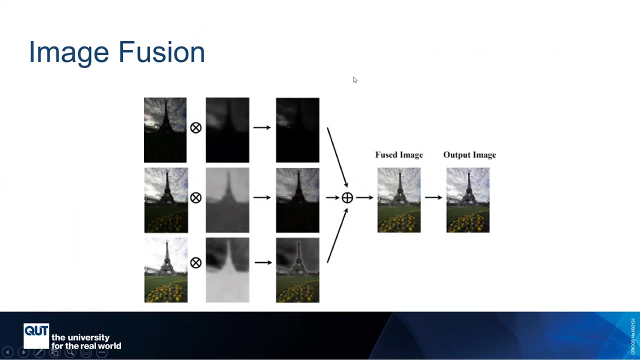 like SVM, KnifeBase, KNewsNeighbor and so on. That's can help in terms of Extract different features from different models to train these classifiers. Type of another type of called image fusion, where you do, for example, segmentation or 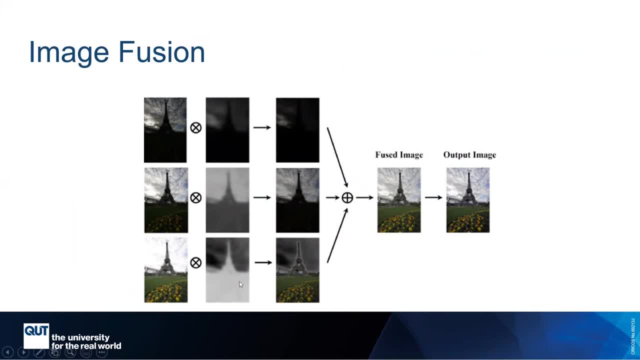 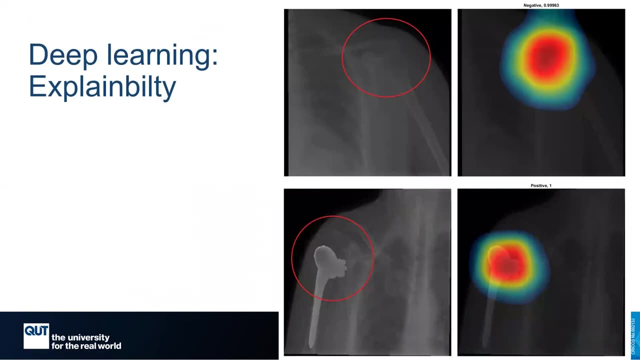 localization or distinction from different algorithms and fuse them in one output image. Could be some of them, not all of them, perfect. However, when you combine them, you get a good image, as you see here. Last but not least, Then, the final thing I would recommend for medical images is deep learning screenability. 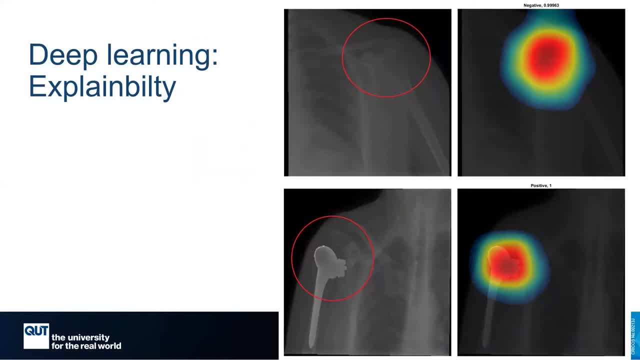 You need to explain. There are several tools, ways and you can come up with a new way to explain how the performance. Usually people think or say deep learning is a black box There is. we don't know exactly what's going on inside. 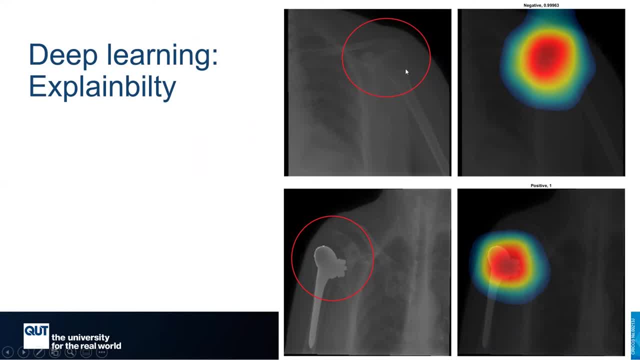 So this is an example showing that where there are ideologies on, the clinicians look at that in order to make the decision, For example. on the other hand, there is a pro of showing the sample- testing samples- where the neural network is looking to them and make this decision. 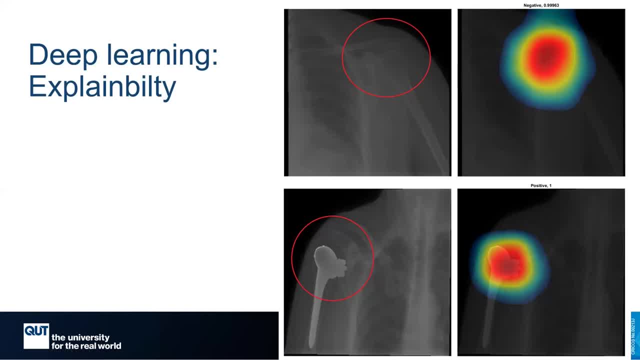 So that's really important part in every single application of deep learning. If both of them- the specialist, the expert and the deep learning models- looking at the same place, then the models work really good Sometimes. By doing that You will figure out the problem. 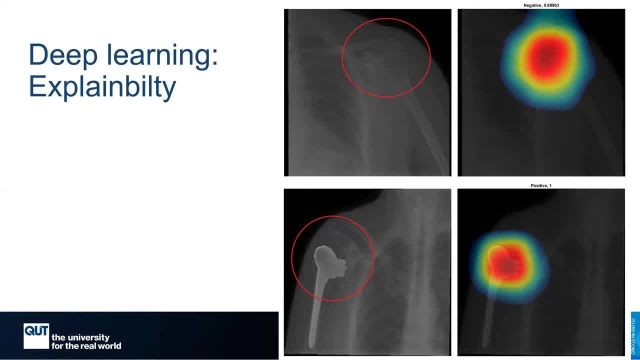 Like. imagine the scenario with whereas a dog with the right background and the cat with white background, and the model is just looking at the background and will specify that the red color is the dog and the white color is the cat, and you will get high performance. 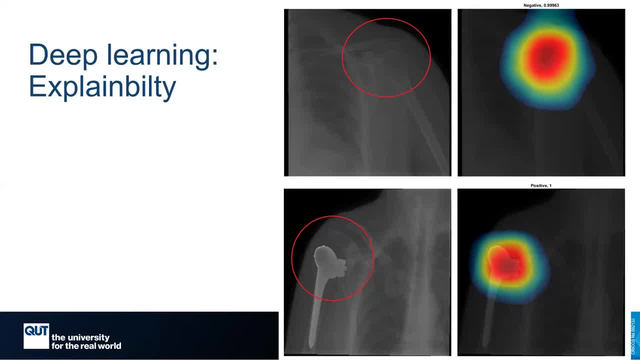 That's really great And you move on. If that background later on changed, the model will give bad performance. So by doing that visualization, All that, That type of tools, You know exactly where the model is looking. did the model extract the right features in? 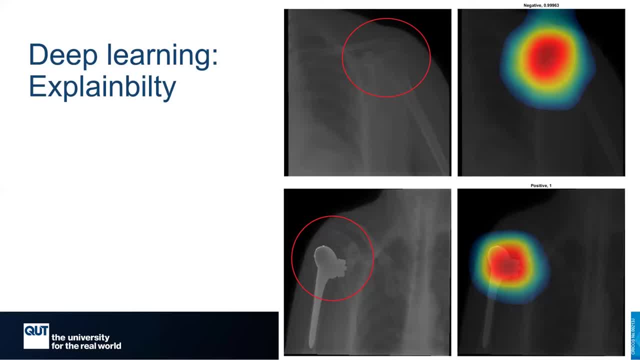 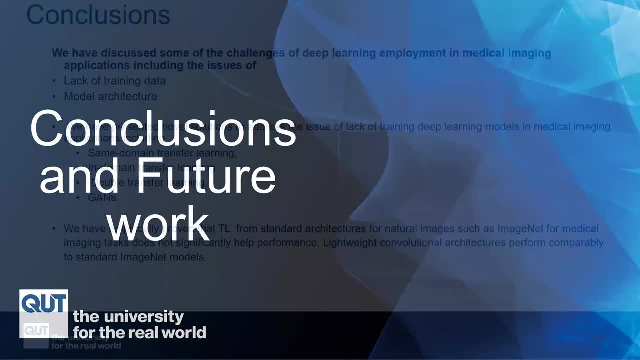 order to make the decision. We're running a little bit low on time now, So I see you just wrapping up now. Yeah, I'm done. Okay, Yeah, So the final thing: we went through different topics like the transfer, learning and data. 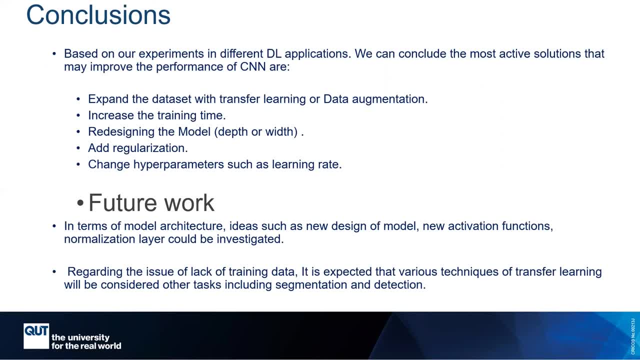 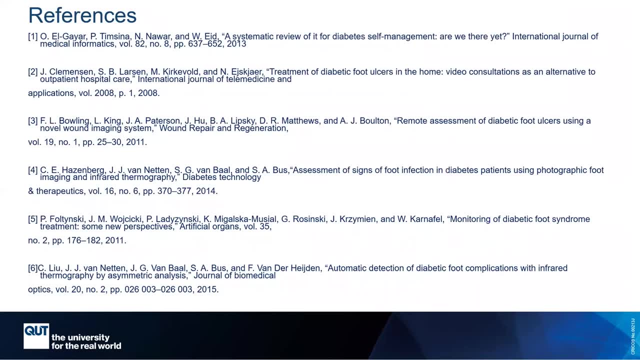 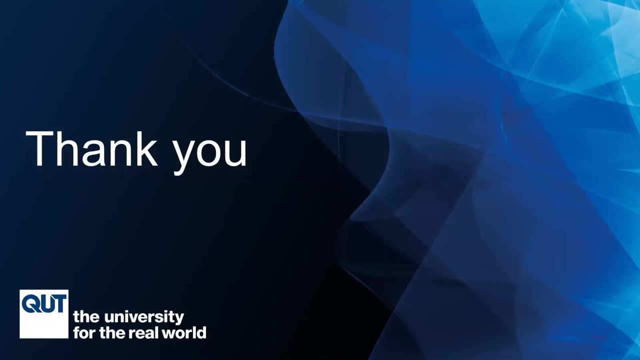 augmentation and even the design I would recommend for the future, like to dive in transfer learning. You don't need to prepare high amount of data, maybe small amount of data with the transfer and we'll show the performance. and thank you so much and sorry for taking that. 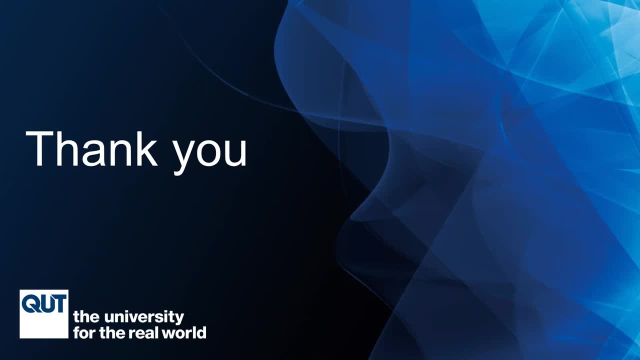 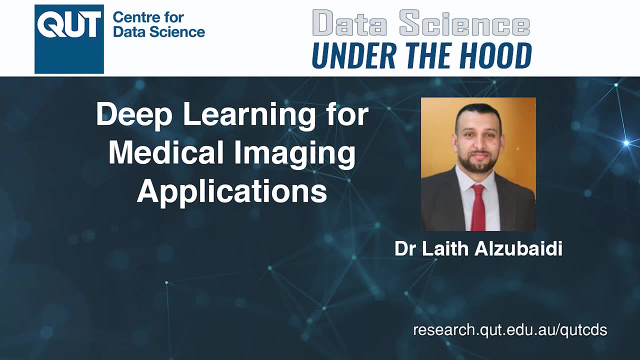 long, It's okay. Thanks, That was a really interesting presentation, So I think we can just sort of dive straight into the questions now. So one of the questions is: for large data sets, how is the class label attached to each image? 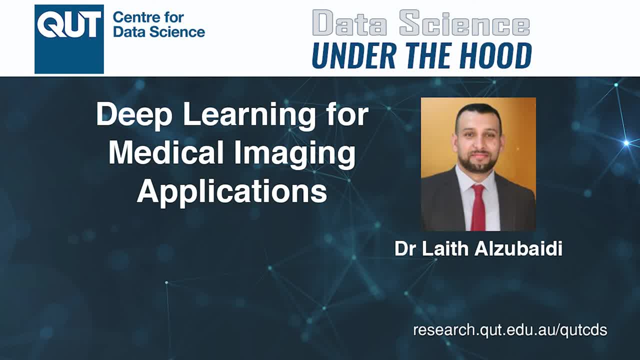 For that, Yeah, So for that, definitely for the target data. for any data set, there is a label for a bunch of images. You don't need to go through one by one. For example, imagine different scenarios of dogs, then all of them are dogs. 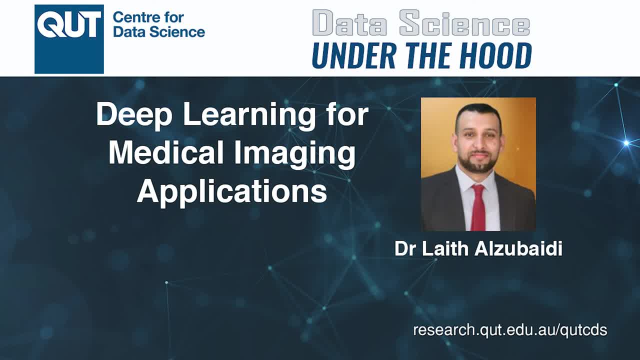 So a whole folder with a million of images. you just sign it a label of dogs. that's all we need For medical images, for example. normal, abnormal. there is one folder of normal, one folder of normal. You don't need to go through one by one and assign the label. 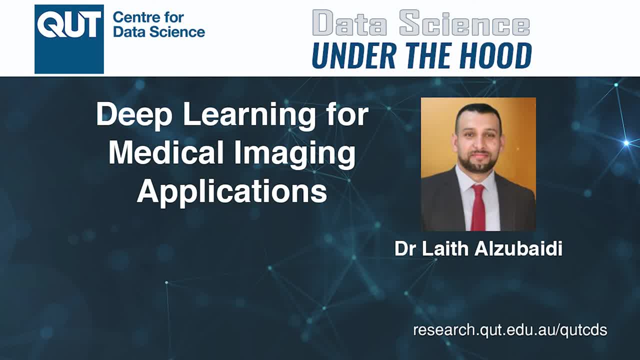 So if you upload these two folders to the deep learning model, we'll recognize that whatever on that part or that group will be normal. whatever on that part will be abnormal. So we don't need to go through each of these images in order to assign the label. 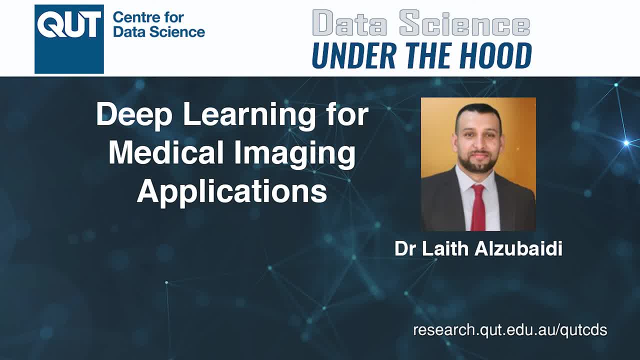 Yeah, Thanks, I think that definitely makes sense. So the next question is: is it possible that images may belong to more than one class? So, for example, in an X-ray it may show cancer, Cancer and a fracture. Is that possible? 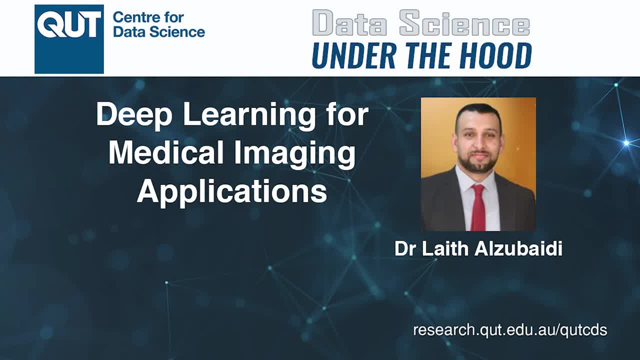 Is it possible if the labeling stage is wrong? That's why we say that we need an expert to confirm the right label for each class. If you give bad class or bad label, I mean wrong label. definitely the model will learn that as the wrong one. 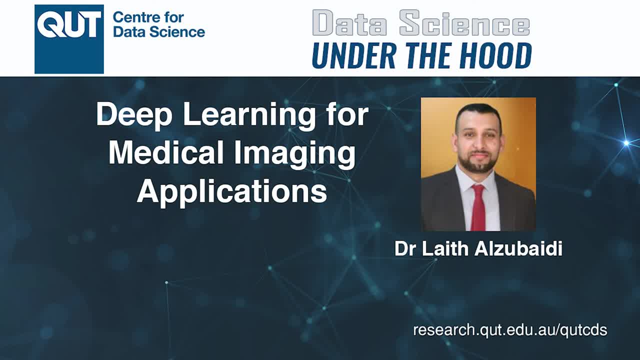 Usually the labeling should be done by an expert to make sure this belongs to the right one. It belongs to the normal and abnormal. Usually they say: if you give the model, trash in, trash out. If you give bad label, definitely you get bad performance based on that. 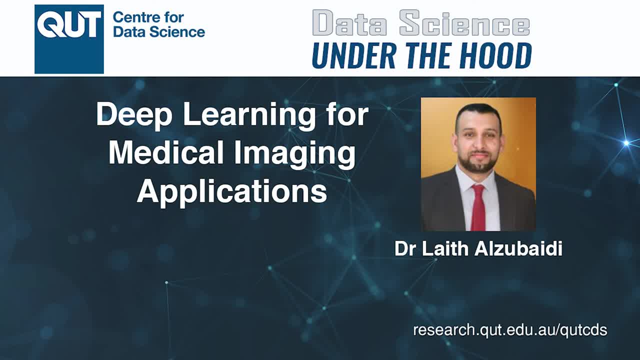 Some of the samples that I experience. we do usually if we have similar stage, we are not sure if that image will belong to any class. We do something called suspected. We do 100%, for example, normal, 100%, abnormal. 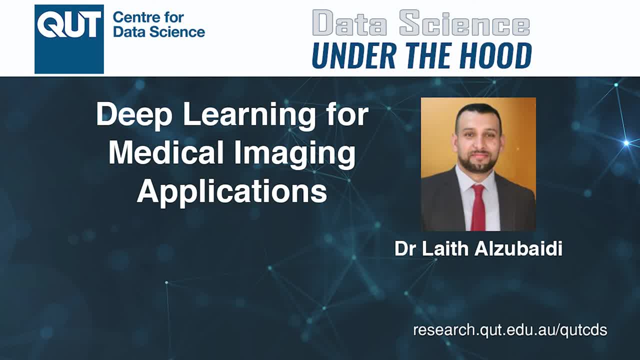 If there's something in between we do abnormal, We do another class called suspected, which is that kind of could be normal, could be abnormal, which is sometimes even hard for the people who are specialists to classify them, Then definitely the model is not able to classify them in the right way. 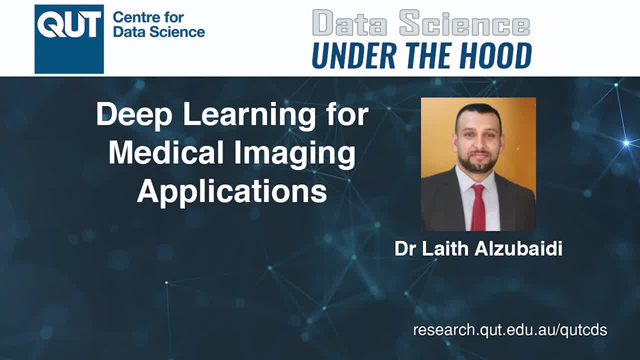 Excellent. So I just want to see if I can fit in a quick question. So I was sort of interested in the transfer learning material. So is there any situations where You might get worse performance with transfer learning? So, for example, if the source data was too different to the target data that you end? 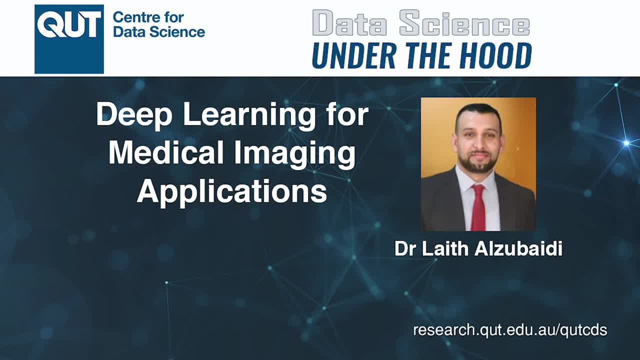 up getting a worse performance And if so, is there any ways to sort of overcome that? So one of the scenarios we experienced, that training from scratch is similar to the training from having the transfer learning from different domains. So I think that's a good question. 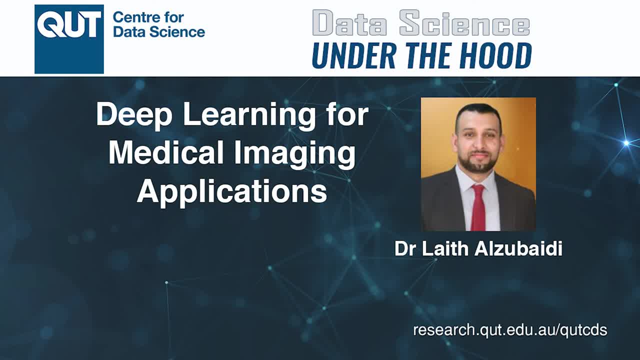 Yeah. So what I see is that the source data is trained from different domain, or sometimes even worse, And there is a paper just published by Google. They showed that a Sholo model trained from scratch on medical images is exactly a little bit better than the retrained models of ImageNet that are trained on different domain. 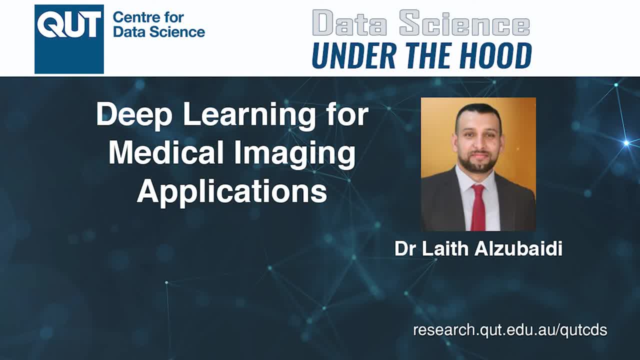 So that's one of the scenarios that I experienced. If you don't have the source or similar source, I would maybe try to train from scratch on this model. we're trying that pre-trained model of imaging it. we're trying to classify 1,000 images, 1,000. 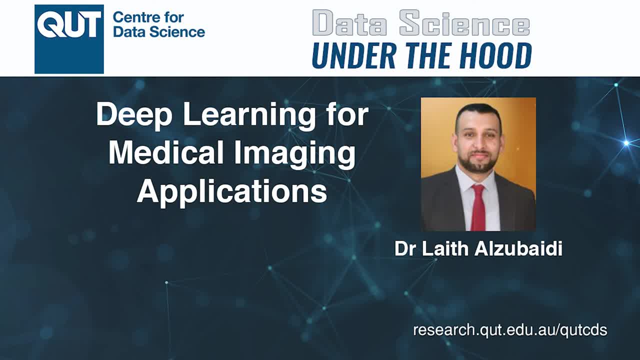 class with 14 million images, so they design were designed for a specific type. however, for medical images, sometimes we don't need to take that very deep models. sometimes a shallow model can help with a few samples of transfer learning from the same domain. definitely would help, even with a. 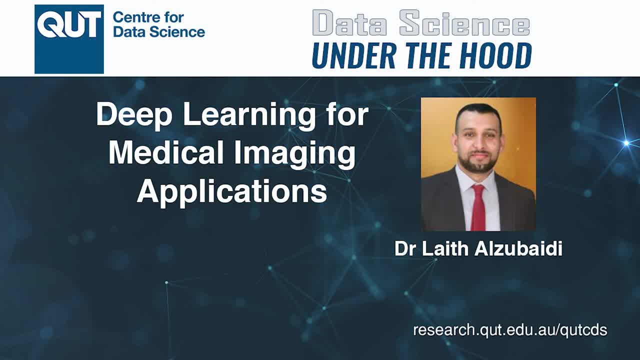 little bit of a cross-domain. we have used, for example, white blood cells to prove the performance of red blood cells. at least they share something, at least they share some of the ideas or some of the features between two tasks. excellent thanks very much. late, so, um, we're out of time now, so 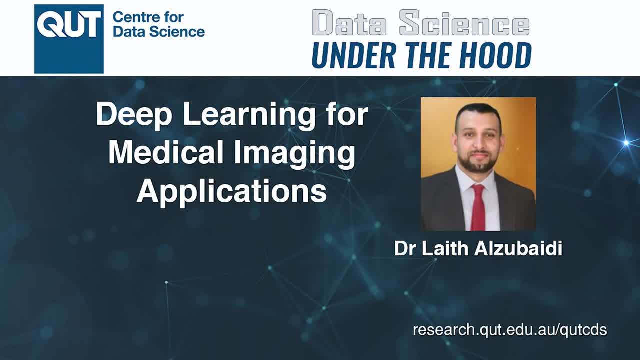 let's bring the session to a close. so thanks very much again late for the very interesting presentation and thanks very much everyone for joining uh. hope to see you next time and bye for now, thank you.